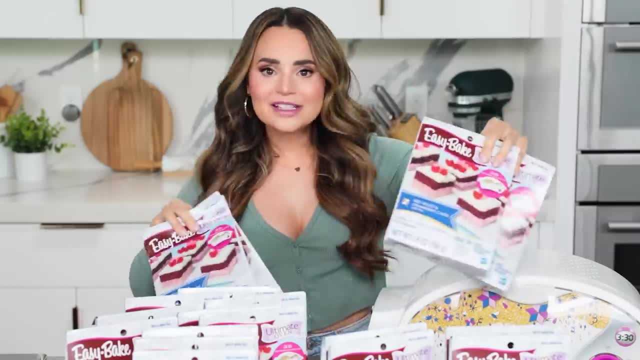 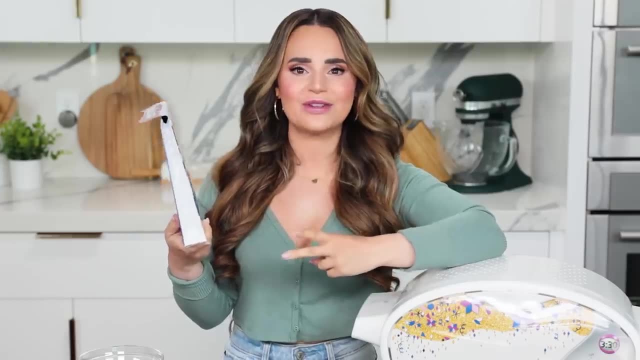 It's a. I got a lot There, a bunch. Here we go, here we go. I got all these cake mixes, You know, at weddings, where you are gonna pick your favorite cake flavor. Well, um, EasyBake only has two flavors, so I hope it's one of the two. 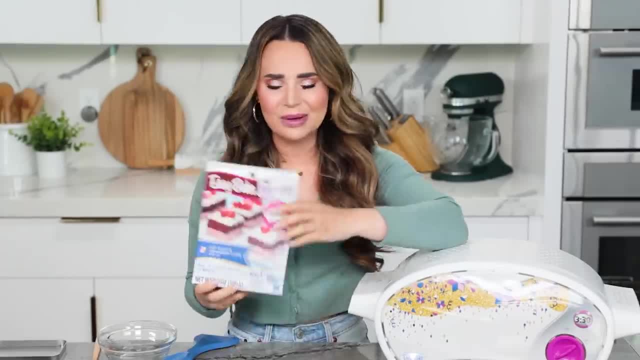 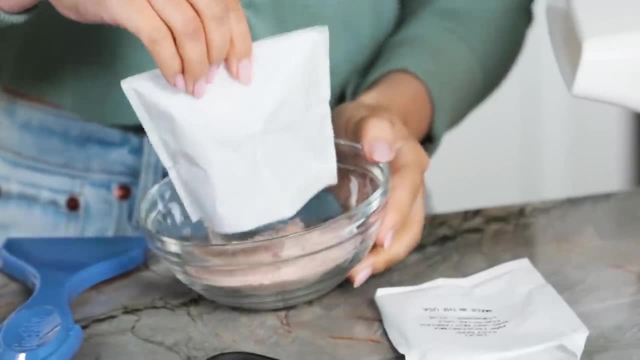 We have red, velvet and strawberry, So maybe I'll make them different tiers or something like that. Pretty easy here. Just we're gonna pour the mix into a bowl. Now we're gonna add 4 teaspoons of water, So this is a two teaspoon. so we need two scoops. 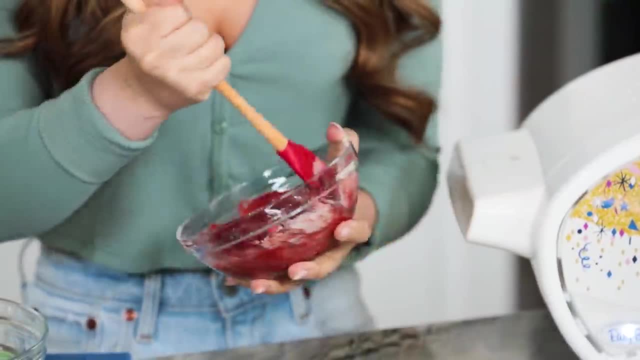 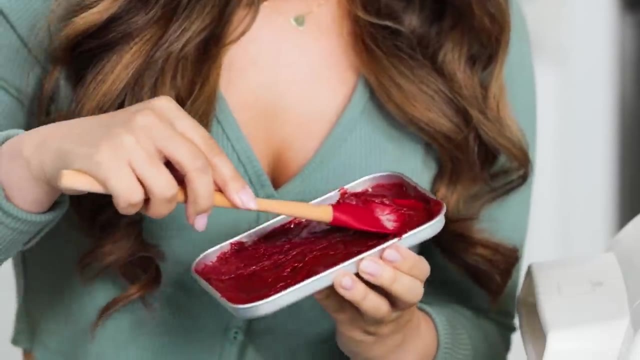 With a small spatula I'm just gonna mix together. Oh, there we go. that's that red velvet cake. Got a greasy little pan, so your cake doesn't stick. We're gonna scoop the batter onto the pan. First cake ready to go. 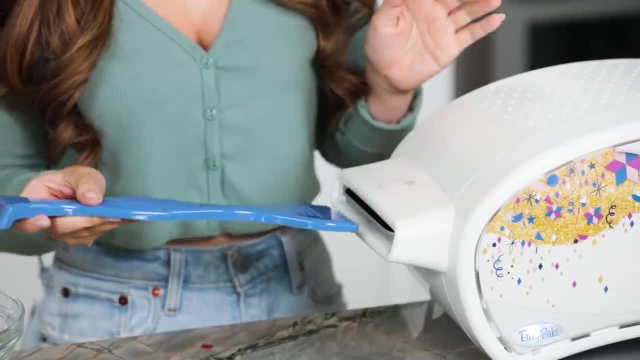 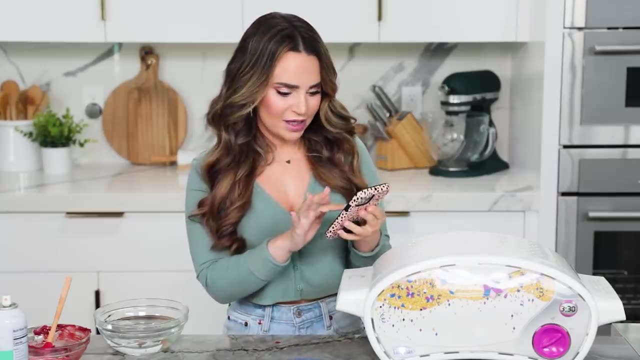 Okay, so I've preheated the oven, I'm sticking it in here and then I press in till here. Now I gotta set a timer. It's gonna bake for 16 minutes and then it cools for five. Oh geez. 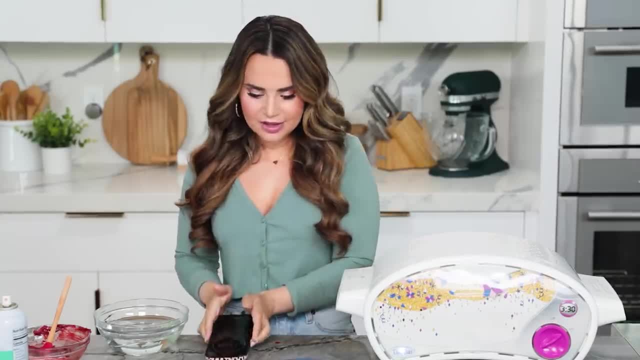 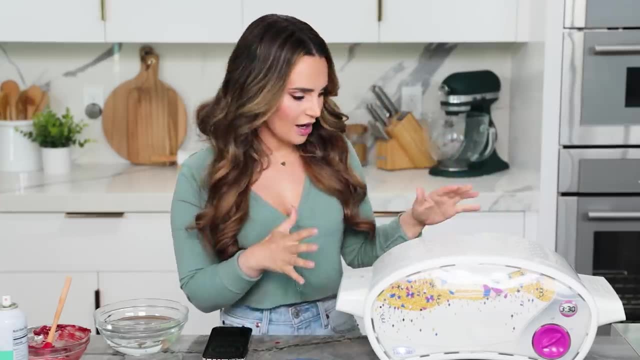 I'm gonna be doing this all day: Start Okay, the timer is going and while this is cooking, I'm actually I'm gonna make more batter, but I'm also gonna get some more Easy-Bake ovens, because this is gonna take me forever. 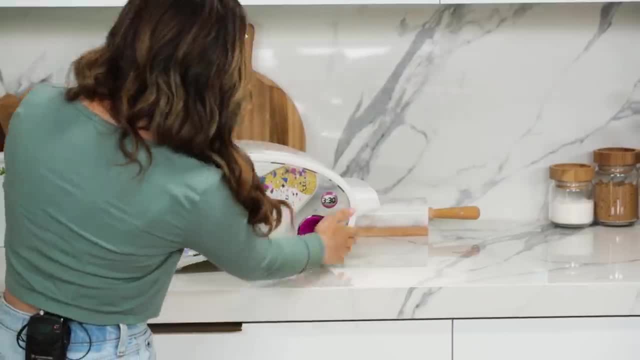 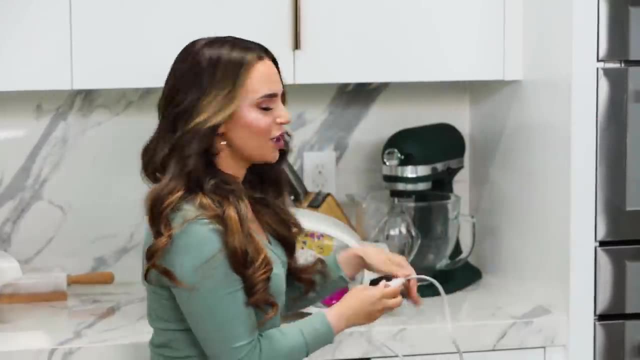 Okay. so let me go get some more. Let's plug these in. Okay, that's on. Oh my gosh, I feel like I'm opening a bakery, like I'm getting my Easy-Bake oven commercial kitchen going. I'm gonna get efficient. 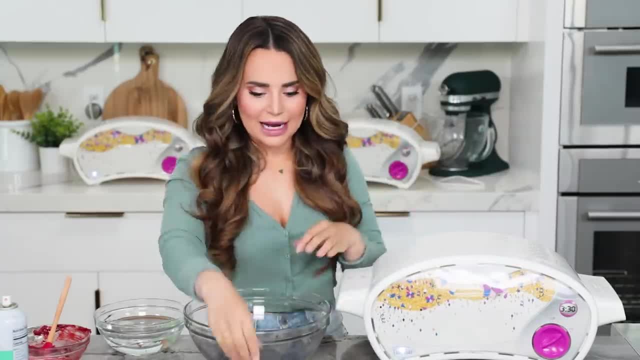 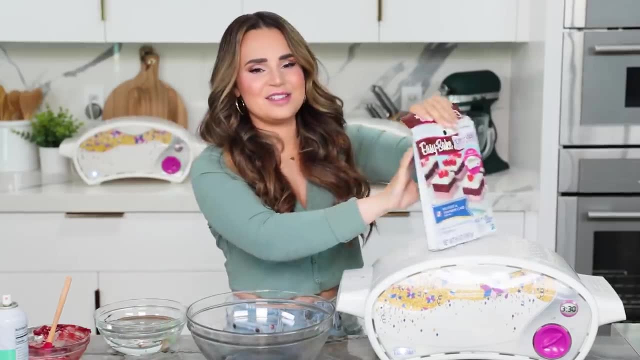 I'm gonna get a big bowl and I'm gonna come up with a recipe. I'm gonna combine multiple packets Strawberry, red velvet frosting sprinkles. I'm gonna open them all up- Red velvet strawberry. There was nothing easy about this. 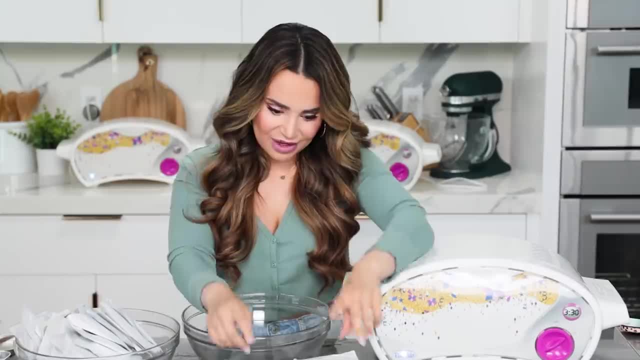 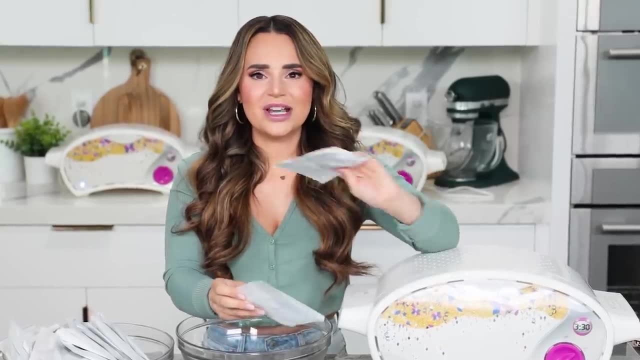 All right, everybody, let's do some math. I've got 19 packets of red velvet cake mix. They each need two teaspoons, so that's 76 teaspoons, which is a cup and a half. Boom, we need a cup and a half of water. 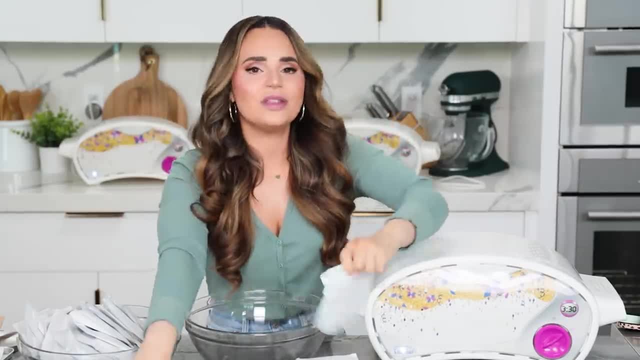 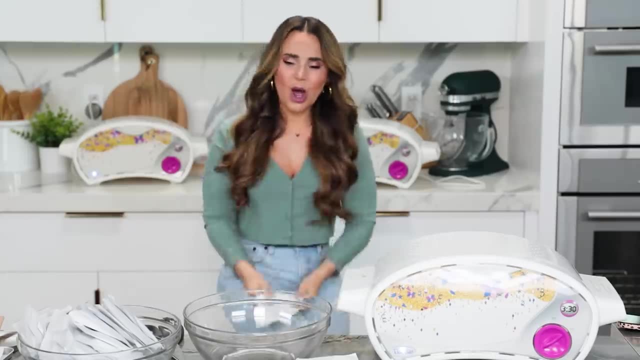 for all of these packets. Let's do that. first I'm gonna open all these, get all the cake mix in the bowl, Then we need a cup and a half of water. That's why baking is a science. Boom, a little math today. 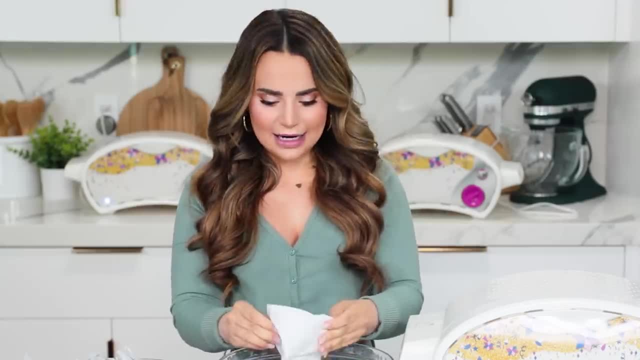 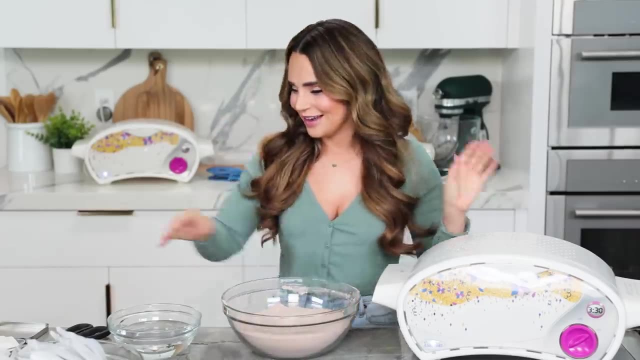 That was a lot of math actually. I wasn't thinking I was gonna be doing that much math today. Let's get these going. Look at all this holy smokes. This is the most Easy-Bake cake I have ever seen. 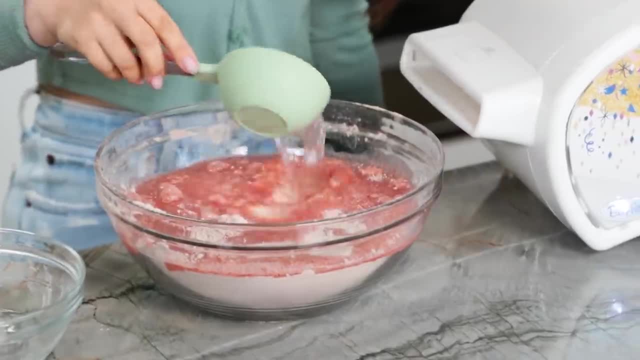 Okay, now I'm gonna add some water. All right, we've got a cup and a half, And I'm gonna keep a little bit more water. Even in the instructions for this cake batter it says that if it's a little bit dry, it's okay. 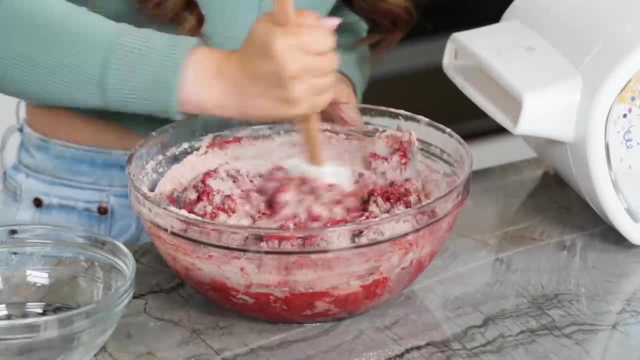 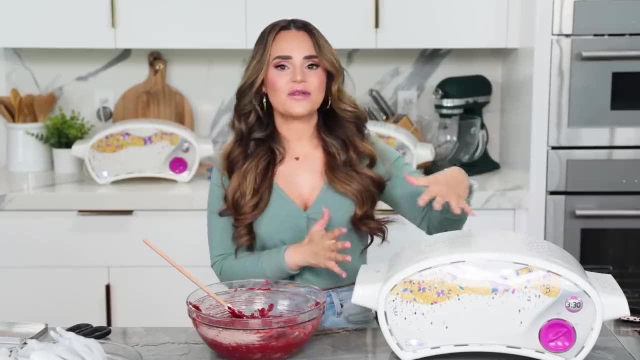 Add a few more drops of water, So in this case I might need to add another tablespoon, but this is looking good. The math was correct. This is looking amazing. Also, our first cake is done baking, and now it's cooling in this chamber. 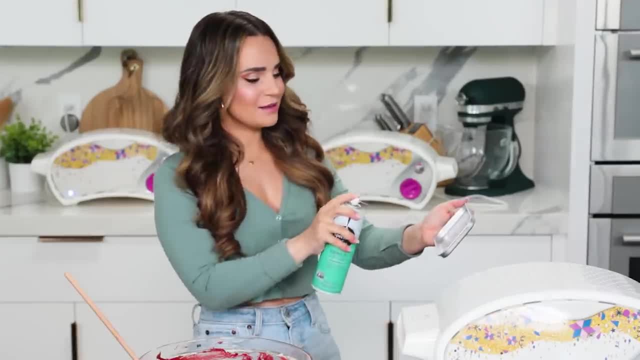 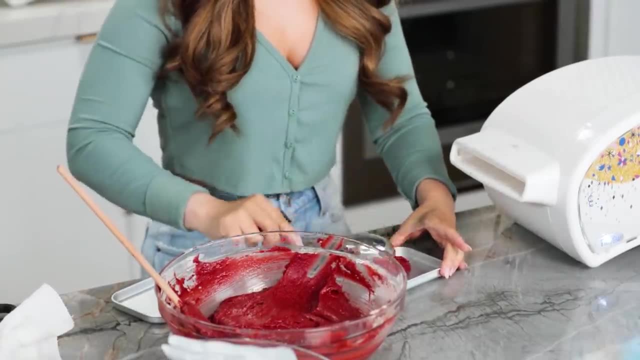 And then we're gonna have our first cake. I'm gonna grease these pans, Spread the grease around nice, and even I'm gonna just scoop batter in there. Every tray's gonna get two scoops, Then you're just gonna smooth it flat. 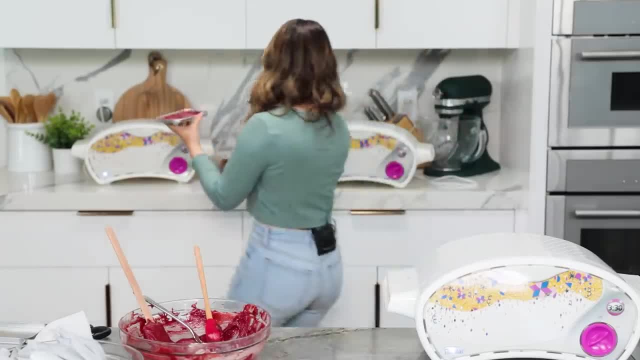 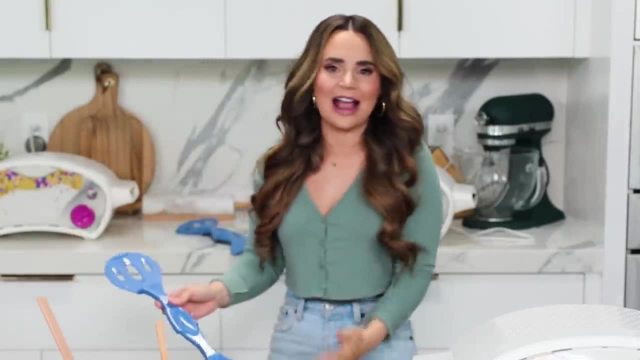 and they're ready to bake. And let's toss these in the ovens. Here they go: One here, one here. Okay, gotta move this down. Oop, uh-oh, Okay, code red, I put them in the wrong side. 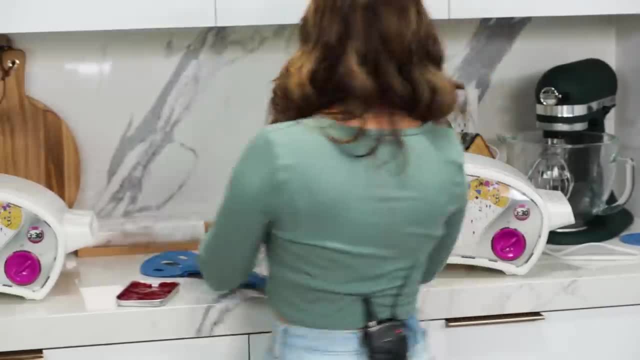 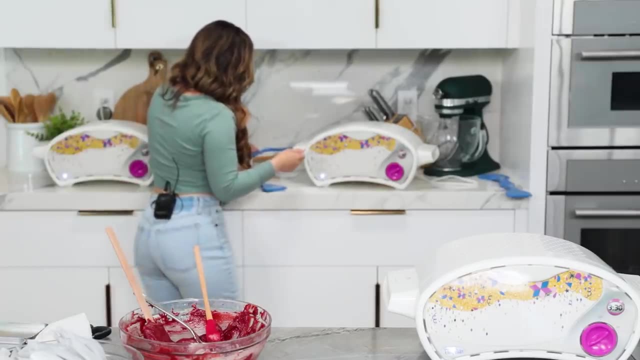 Oh, got it, got it. okay. oh good, This one didn't go in that far. Okay, goes in this side. Oh, my gosh, oops. And then into here. Yeah, cakes in the oven. cakes out of the oven. 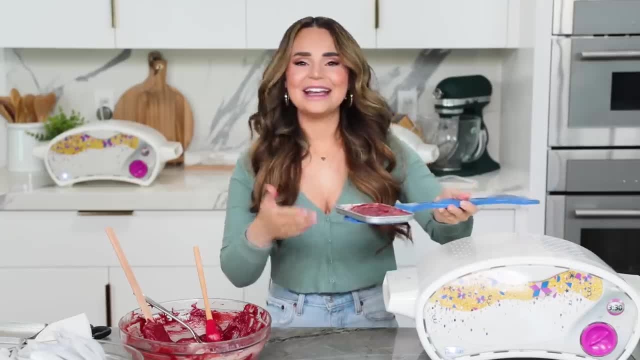 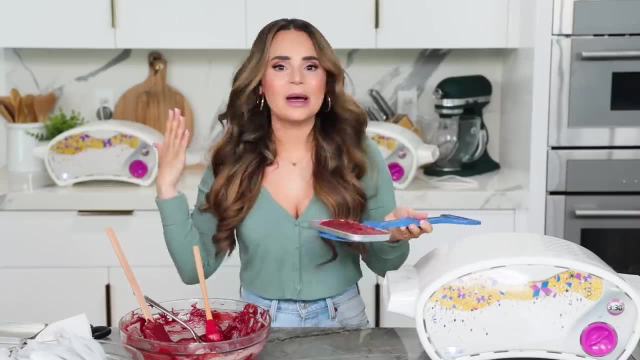 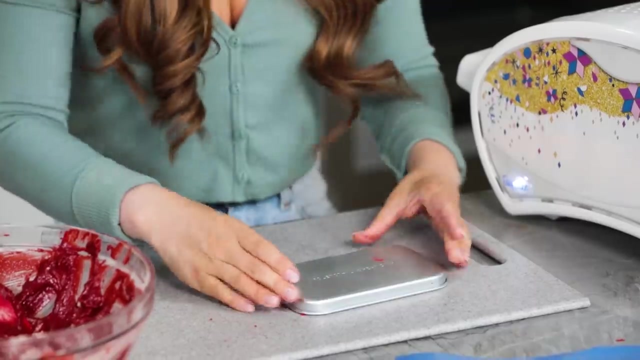 Hot, It's happened. Here is our first cake. It is baked, it is cooled and I'm gonna pop it out of this pan and keep filling these cakes up. I'm gonna put these on a cutting board. Okay, here we go, here we go. 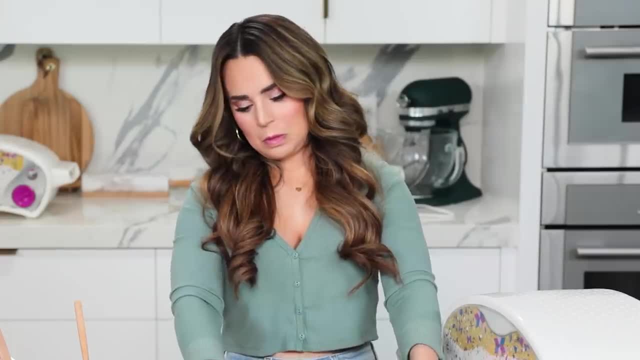 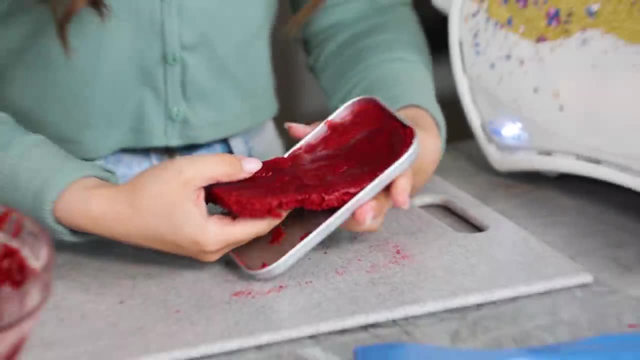 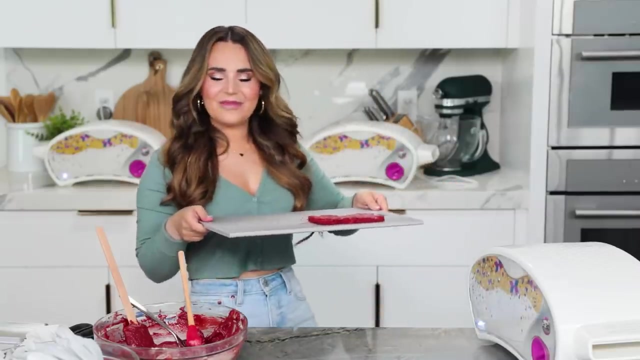 Please be a cake. please be a cake. It's still stuck in there. Oh, oh, oh, oh Da-da. Okay, First cake done, Now just 25,, 30,, 40,, 50,, 60, more to go. 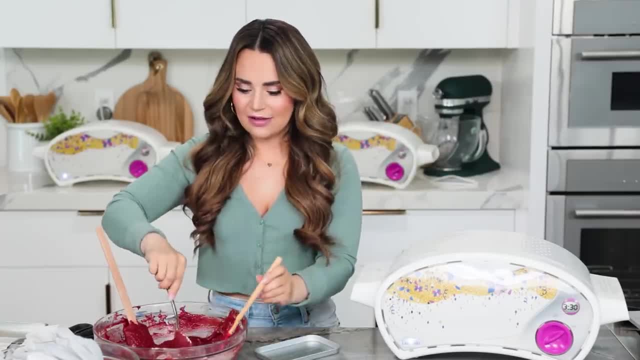 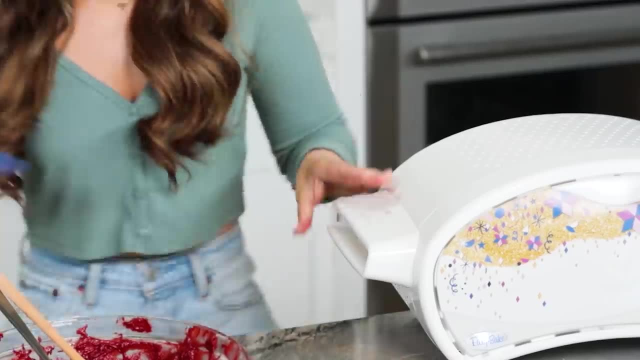 So I'm gonna use all of this red velvet batter until it's gone. I'm gonna get a great arm workout today. Oop, okay, another one goes in. Boom. Just finished baking all of the red velvet cakes. The last few are cooling over here. 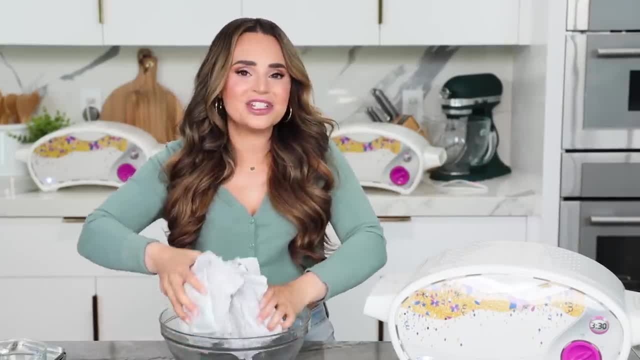 and now I'm gonna start on the strawberry cakes. We have 20 packets. They each need five teaspoons a piece, which is- you know, I don't know, I don't know, I don't know- 100 teaspoons. So that is two cups of water. 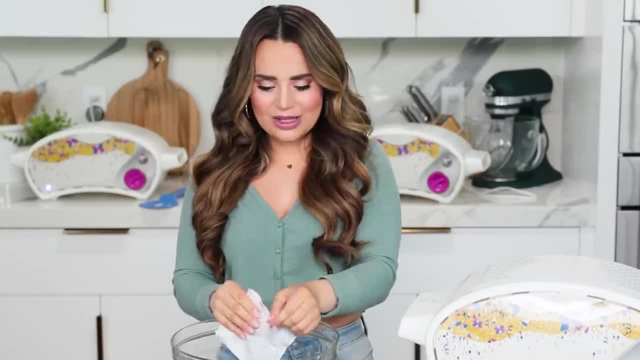 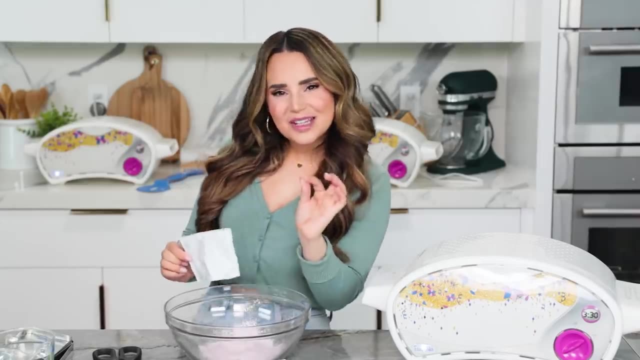 Hopefully the math is right. Whoa, No, we know it's right. Okay, let's do this. Sometimes, when I'm baking, it's about the details, It's about precision and decorating. Today, it's about endurance. This is endurance: training everyone. 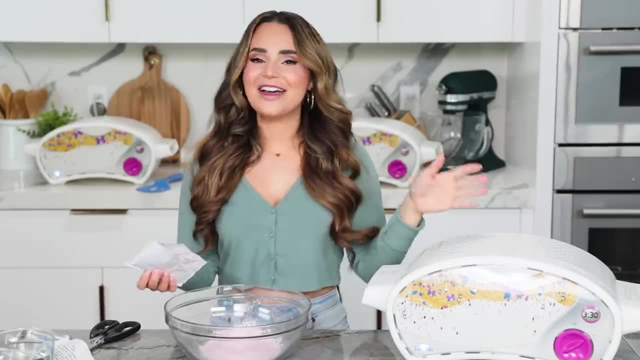 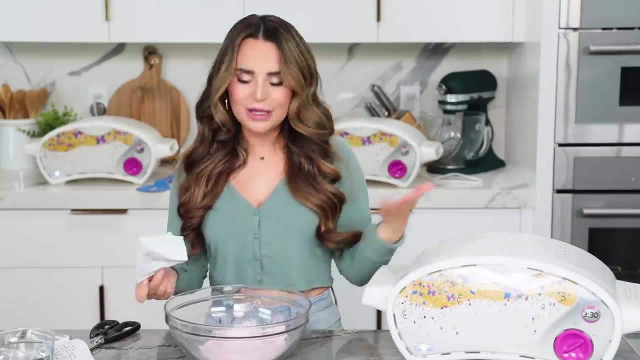 Gotta do a lot of things. a lot of times I've actually gotten a lot of requests to do a 24-hours baking challenge and I think you know it's gonna be a lot of fun And I think I'm unintentionally gonna be doing that today. 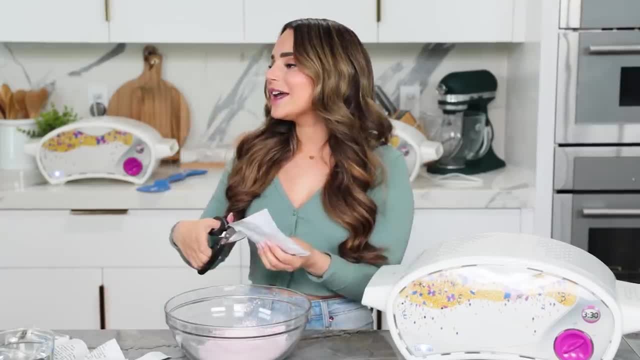 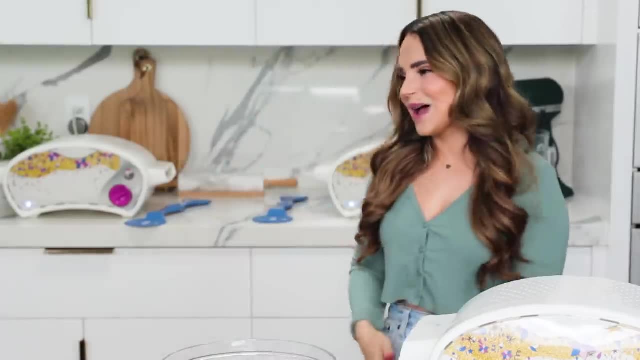 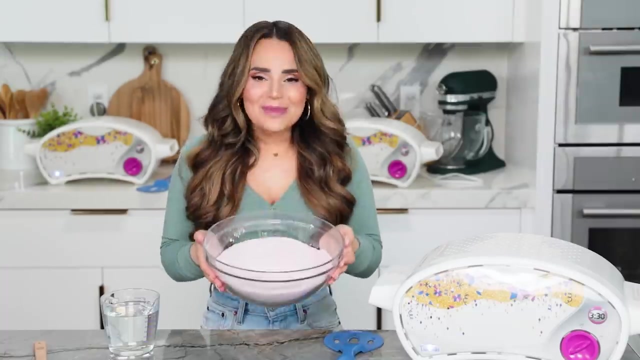 This is gonna take forever. Hey, Mom, We're making a wedding cake today with Easy-Bake Cakes. I didn't know it was possible, Mom, anything is possible. Yeah, All of the strawberry cake mix is ready and it smells like a strawberry milkshake. 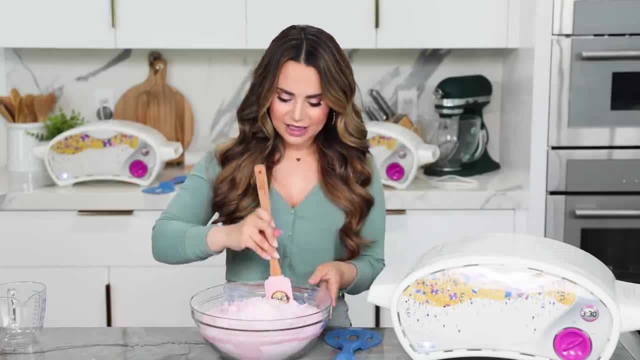 Now it's time we're gonna add two cups of water. It's a different measurement than last time, because for the strawberry packets it's gonna be like I don't know, Five teaspoons, It wants five teaspoons. And for the red velvet cake mix. 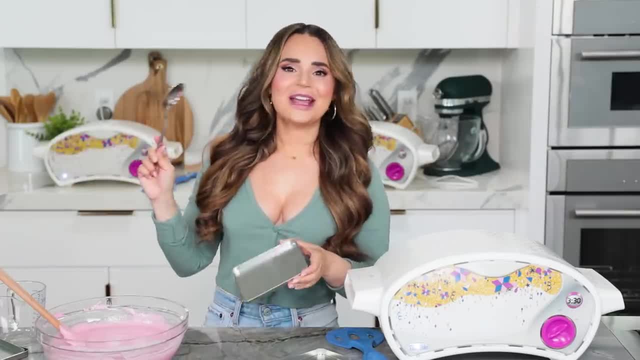 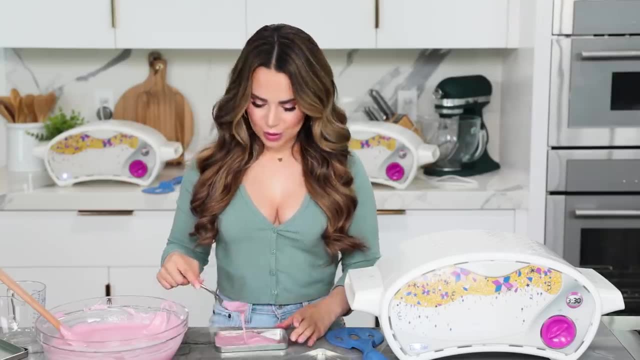 it only needed four teaspoons a packet. All the strawberry cake batter is ready to bake. Gonna scoop again two scoops into this pan. This batter is more smooth. It's a little easier to work with. I really like that. 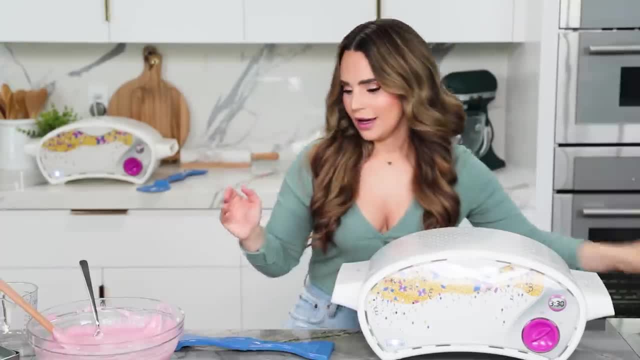 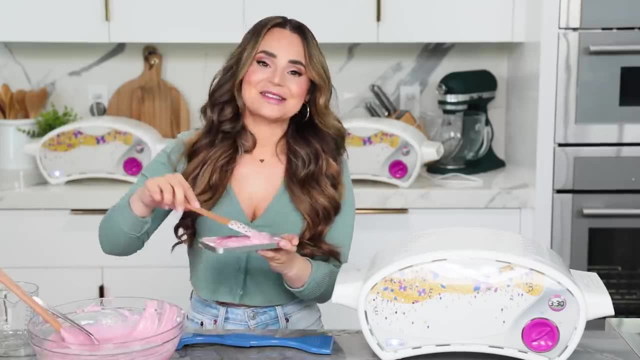 Pop it in here. 16 minutes, boom start. Okay, let's get these other cakes going right away. You guys know the deal. We've got a bunch of these to make, All right, so I'm gonna see you guys in a couple hours. 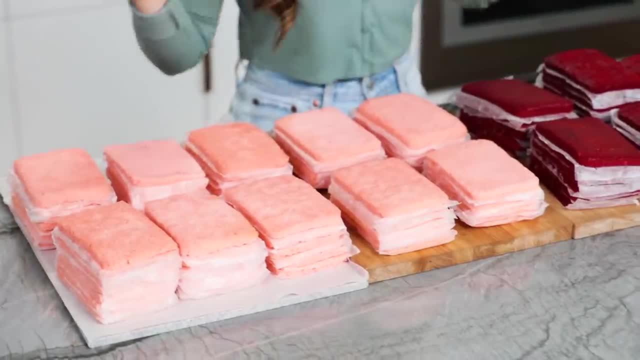 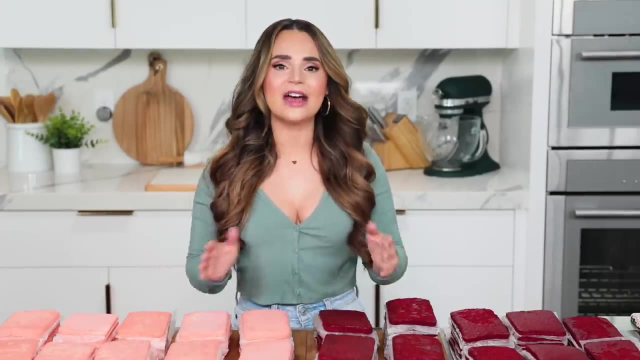 Whoo. So here is all of the Easy Bake Oven cakes that I have made. I have spent my day, entire day, baking mini cakes and I have no regrets. After I bake them, I let them cool, I pop them into the freezer for just a little bit. 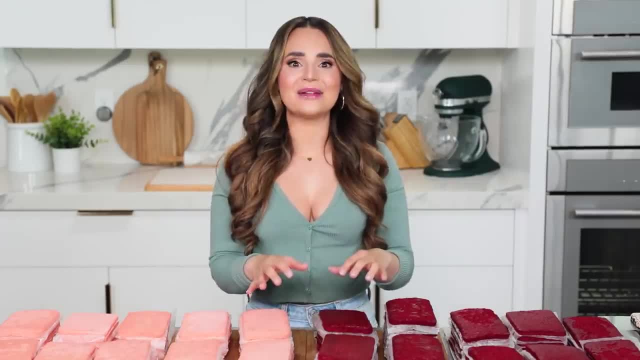 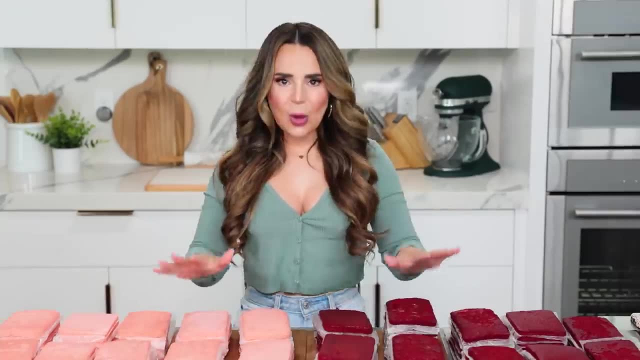 to hopefully make things easier, and now I am going to stack them together, frost them and carve so that they'll look like a cute little wedding cake. That's my plan, anyways. My goal is to make a three-tiered cake. 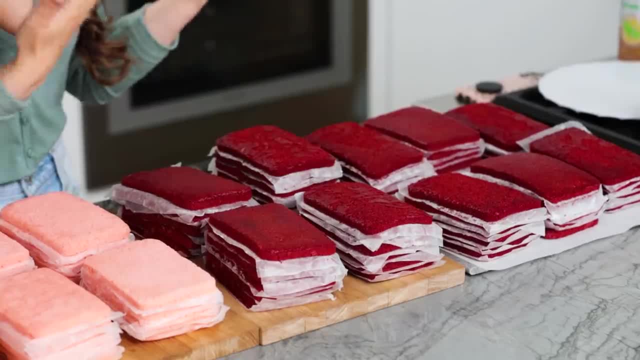 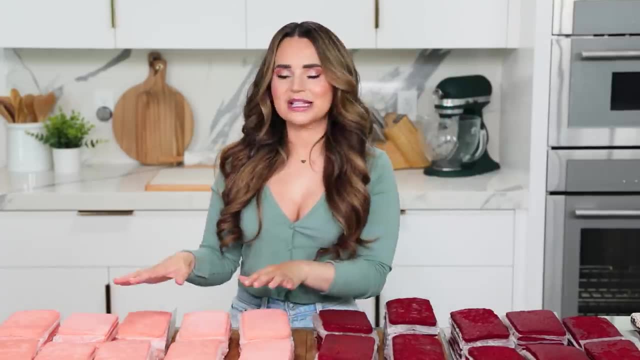 and the red velvet cake recipe seems to be a little bit more dense than the strawberry, so I'm gonna use this one as the base, because that's the biggest cake, and then I might do this for the second tier, Okay, so I'm gonna move some of these out of the way. 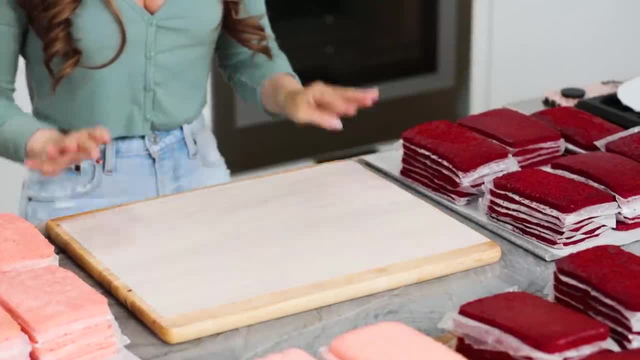 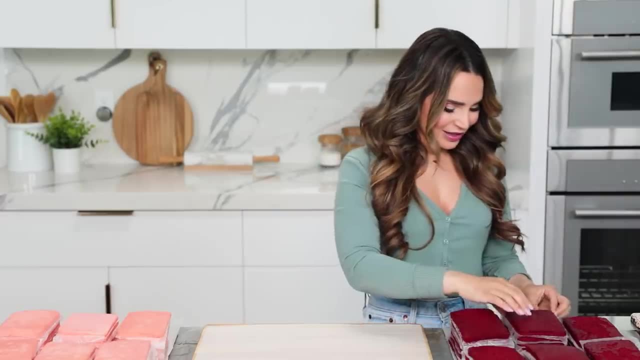 Got a little cutting board over here and I'm gonna put down a piece of parchment paper so that it won't stick. And here goes nothing. I'm gonna take a little cake, place it down and I'm gonna see how many of these I need. 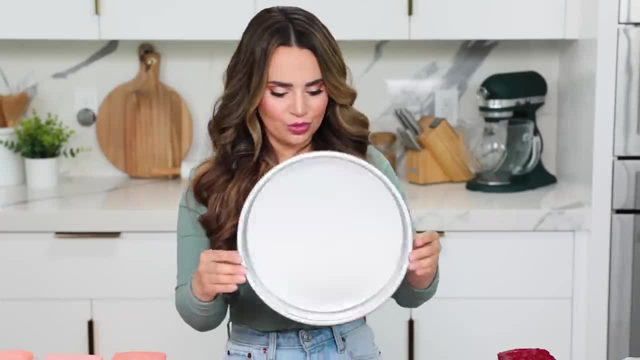 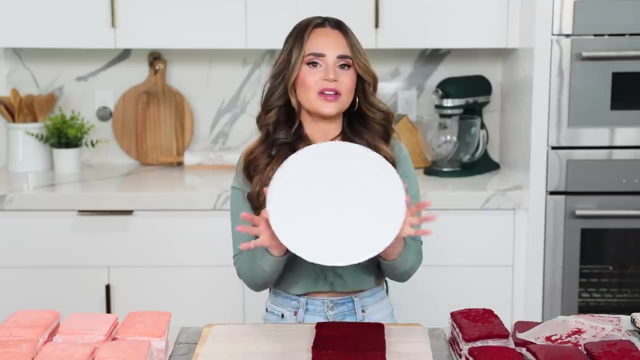 I think I'm gonna have to do this. I think I'm gonna need six. Here's a 10-inch round cake pan- I'm just seeing you know what. Perfect Six as a base and I'm gonna put down a little cake plate. 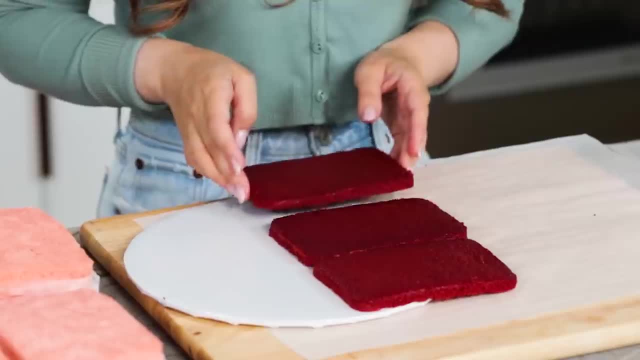 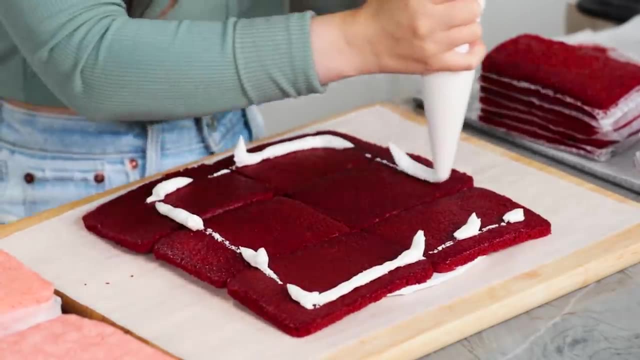 now that I know that's the right shape and I'm gonna layer these like so. Can you see that I've got my first layer on. I'm gonna do a really thin layer. I mean it's like thin little glue just to hold this together. 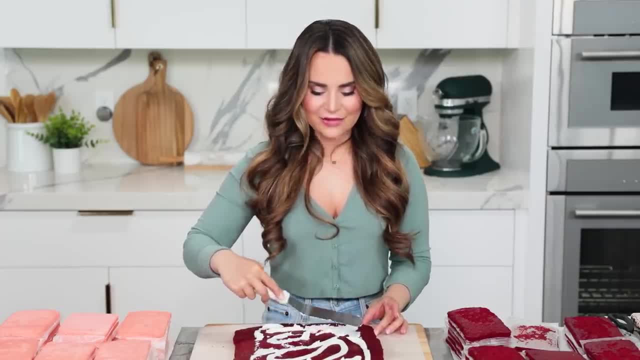 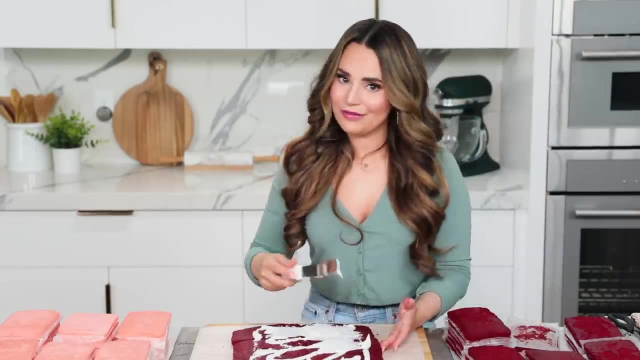 This kind of reminds me of making pedophore cakes. They're these little French cakes that have a bunch of layers. Whoa, even fancier- A pedophore wedding cake. I mean, that's pretty fancy. Now I'm adding the next layer. 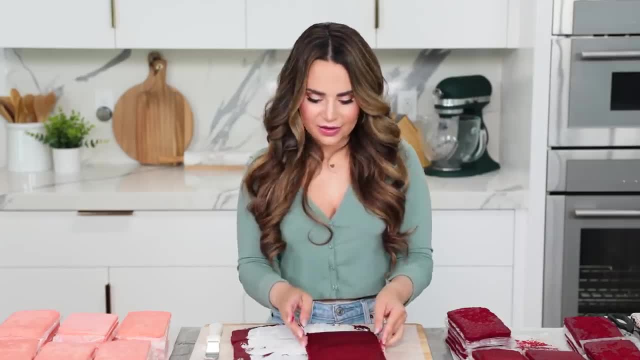 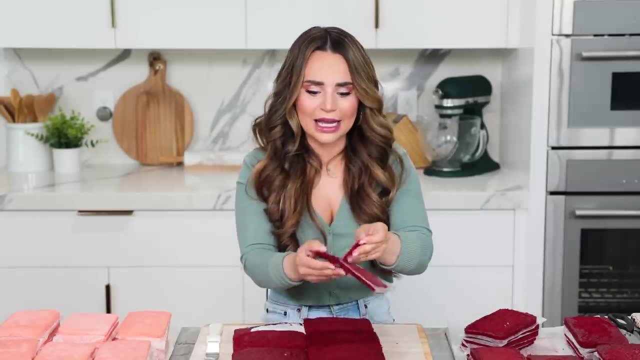 and I'm just gonna keep doing this till I get the height of the cake for the bottom tier. They've only been out of the freezer for a few minutes and they're already getting a little bit softer than I'd like, so I might have to pop them back in. 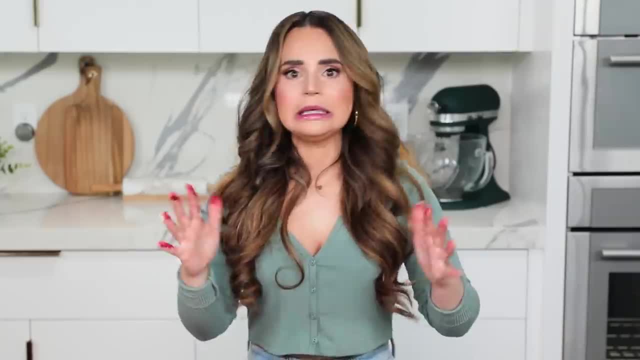 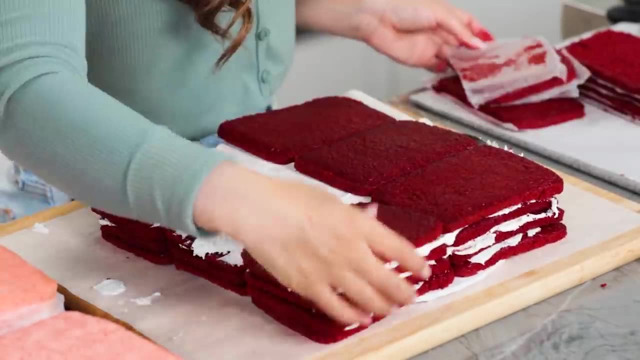 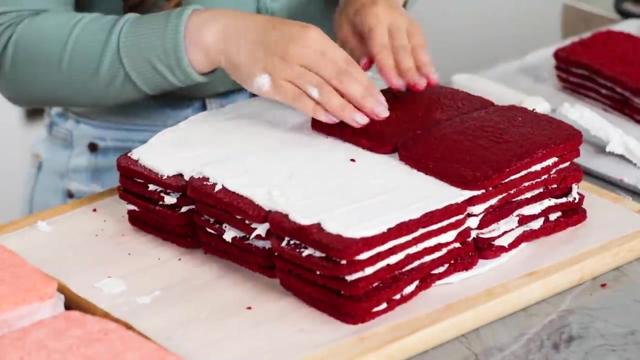 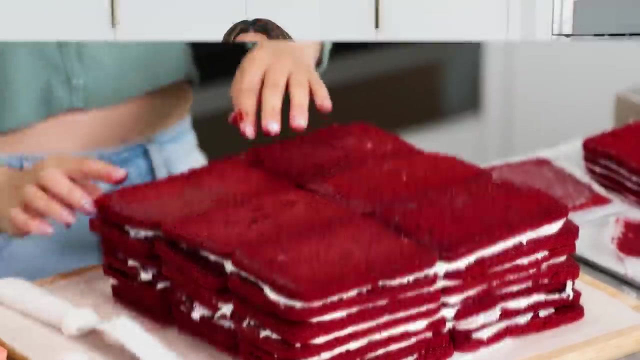 I'm hoping to get this tier done before I have to do that, though, We'll see. Ooooooo, ooooooo, ooooooo, ooooooo. Let's get started. Okay, the first tier is looking good. 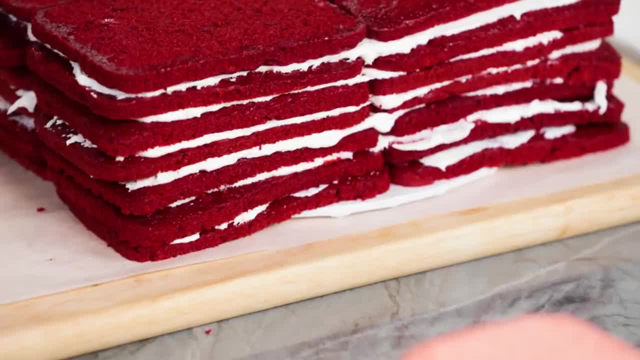 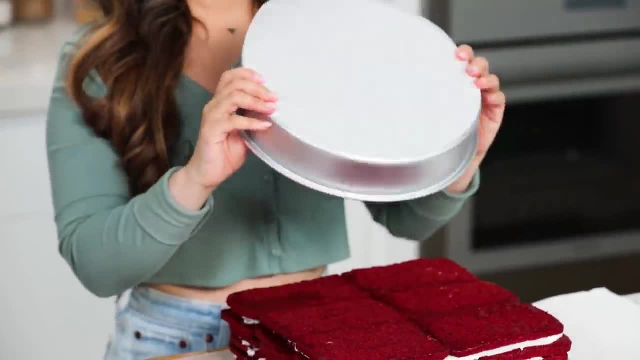 It's more like a pedophore cake. like I said, only a pedophore-. This is a pedo- seven. Wait, one, two, three, four, five, six, sep-, Peta-seven. And now I'm gonna use this to carve out the shape. 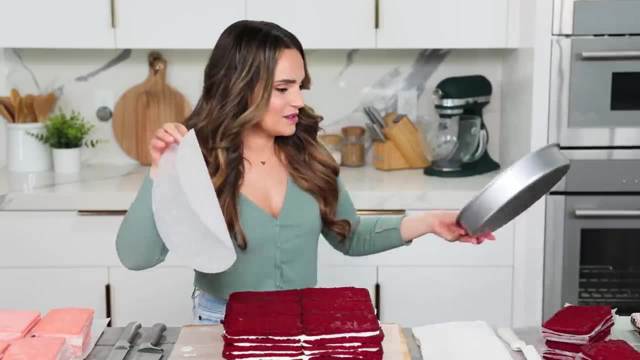 And I've just cut out the bottom of the pan size onto a little piece of parchment paper to make it a little bit easier, So I wouldn't have to carve around this big pan. I'm gonna place it on the top. Oh my gosh. 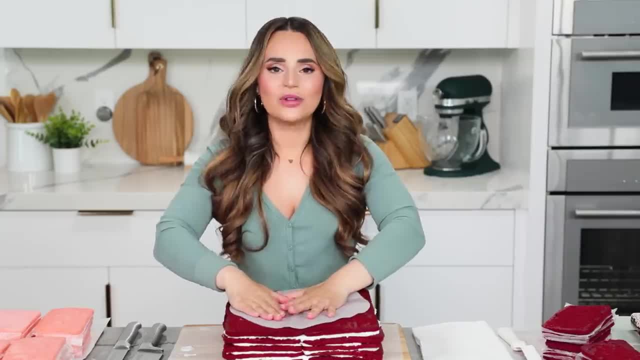 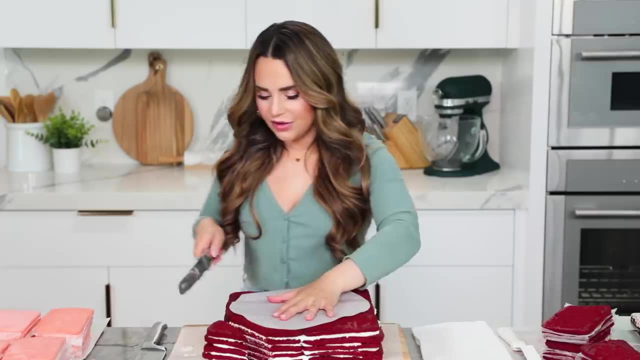 I mean, it just fits whoo. Wish me luck. I'm gonna try to hold this together and hope that the cakes are cold enough to not fall apart. Okay, here we go. I'm just gonna start carving. if you've never carved before, it really helps if the cakes are cold. They're less crumbly. Okay, so far. 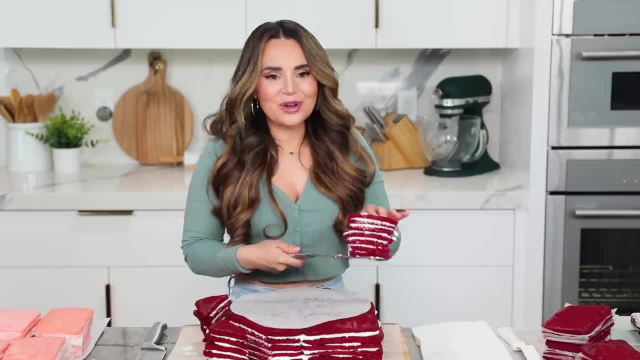 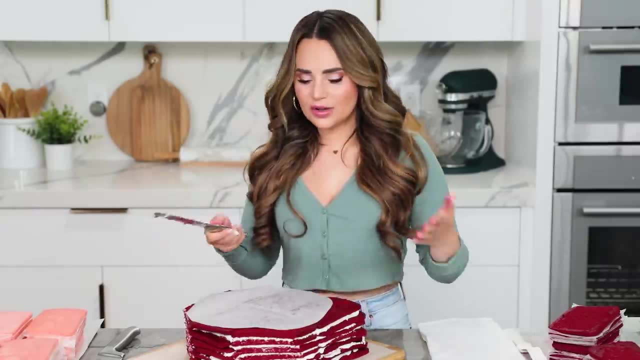 We're holding together. This is good news. and look when you bite in for a slice. Fancy little layers- very decadent. I'm making my wedding cake with circle tears. You can do whatever shape you'd like, but this is how I love wedding cakes. but I've seen people do all, all shapes. 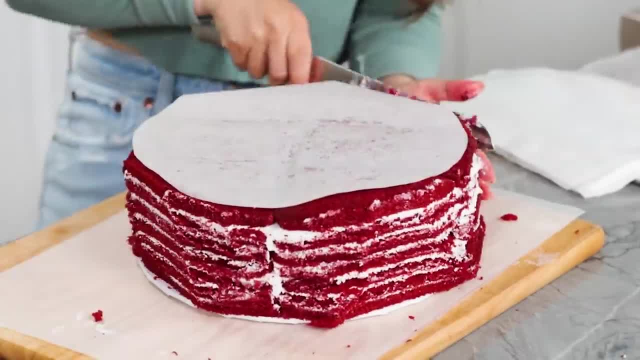 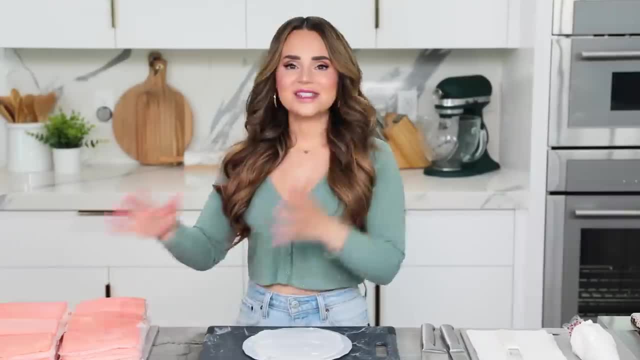 All right, I'm just gonna keep working around trying to make this smoother and smoother. Okay, this is looking pretty good. I think I'm gonna pop this in the freezer while we start our next tier. For our second tier of wedding cake, I'm gonna use the strawberry cakes and I'm gonna do the same thing. 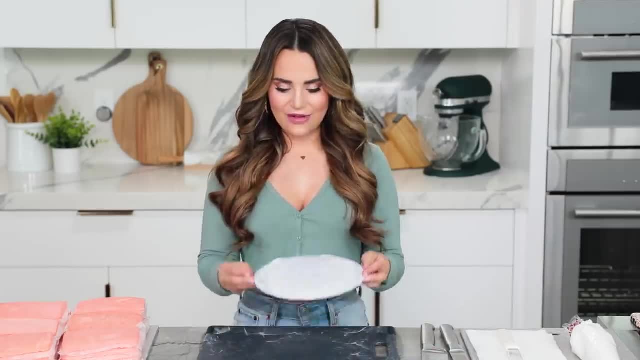 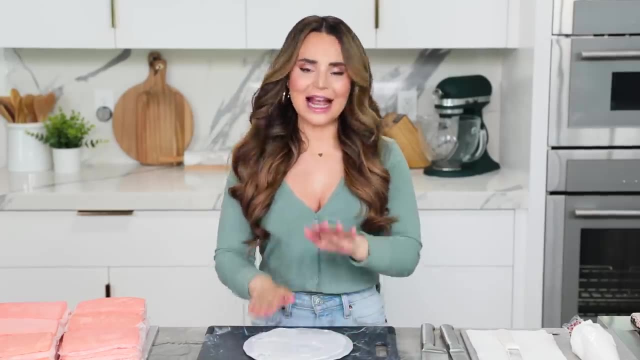 That I did before with the first Here with the red velvet. again, I've got a little cake plate in front of me. It's an 8 inch. I put a little frosting on there, So I'm gonna try once again. I'm gonna stack them up ice in between and then carve. 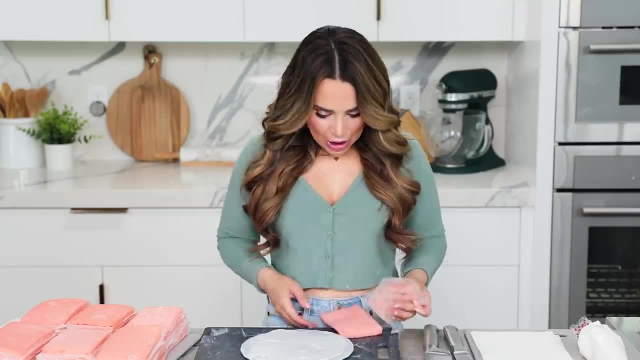 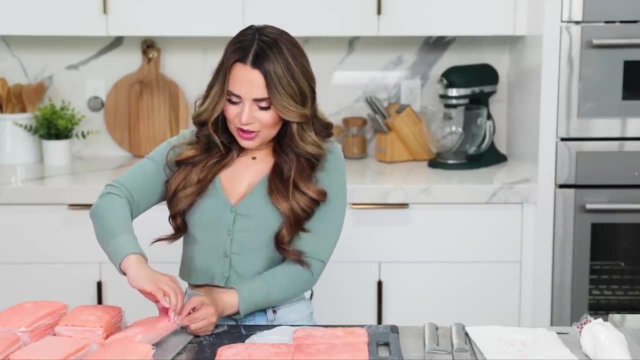 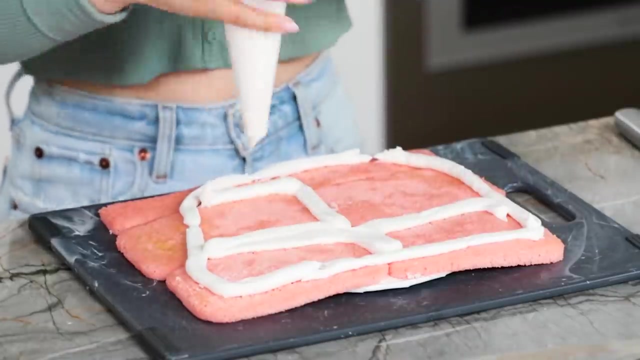 Okay, these are frozen. Oops, let's just stick them right on there. It feels like there's more moisture in this recipe. It's harder to get them apart. They don't like this. Okay, Put a little icing on the top and fingers crossed. these hold together because they are not as dense as the red velvet and they 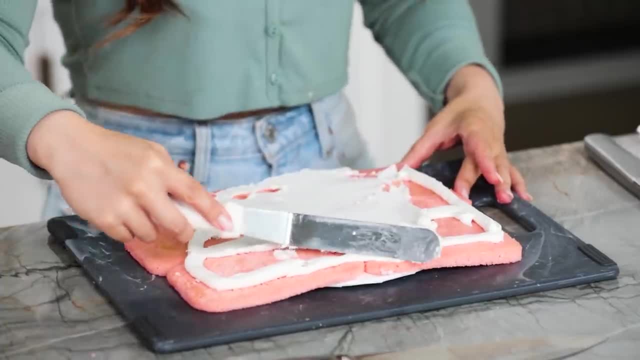 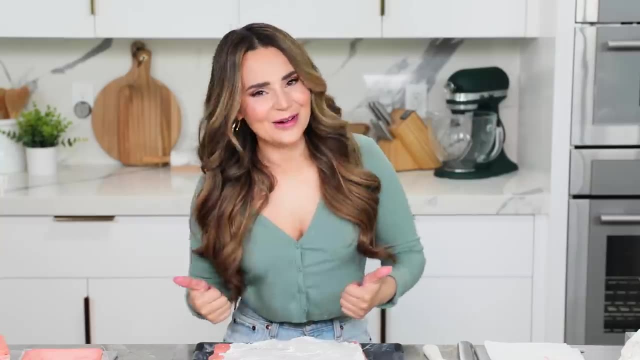 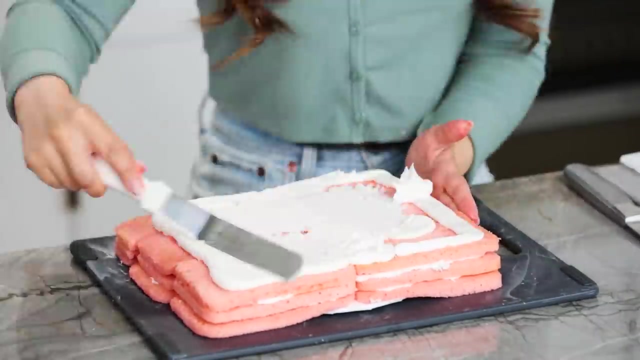 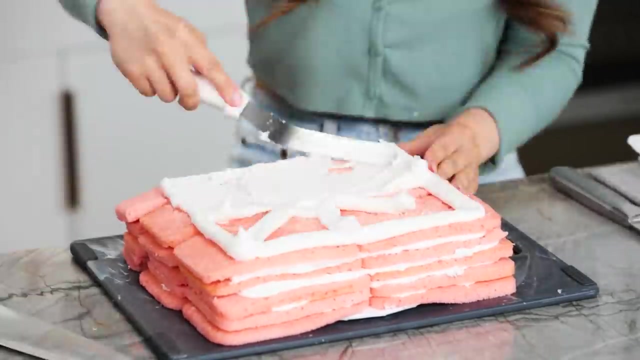 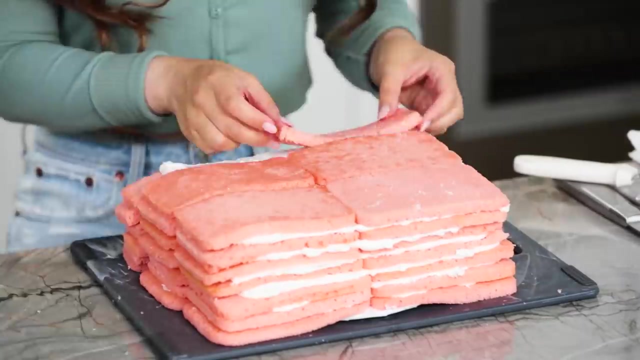 Have a little bit more moisture, They're a little bit more floppy, but they do have a cake plate for support, So I'm hoping that that works All right. only six more layers to go. The pink cake: I'm gonna be honest with you guys, She is a bridezilla. 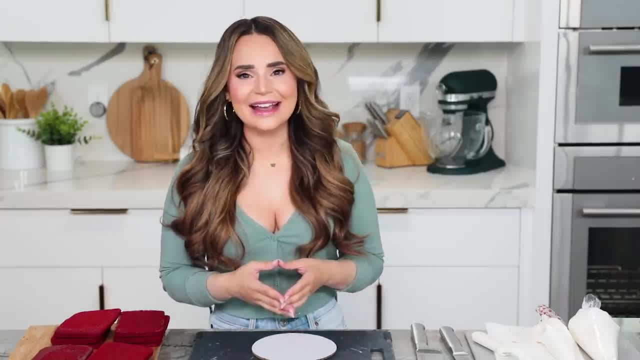 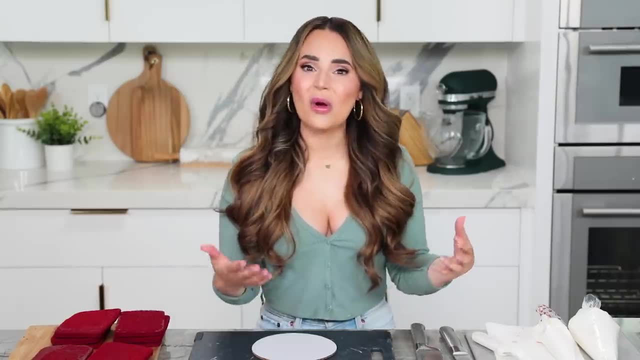 She is barely hanging on by a thread. for her wedding day I had to throw her in the freezer to set up again. There's too much moisture in the cake. It's very delicate. I'm not sure if it can hold the weight. There is a cake plate. 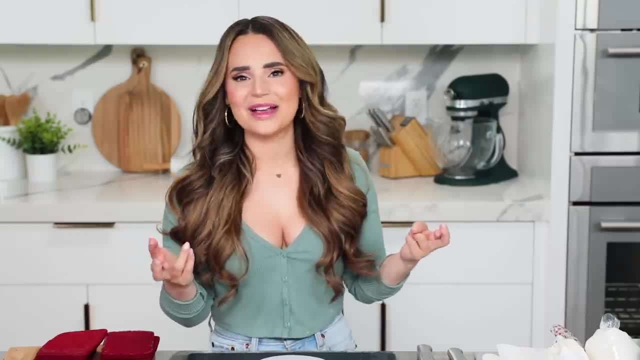 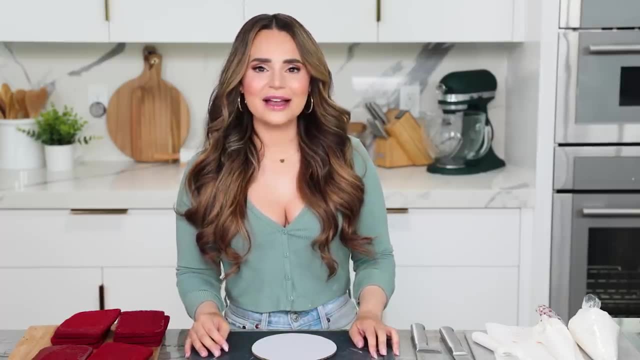 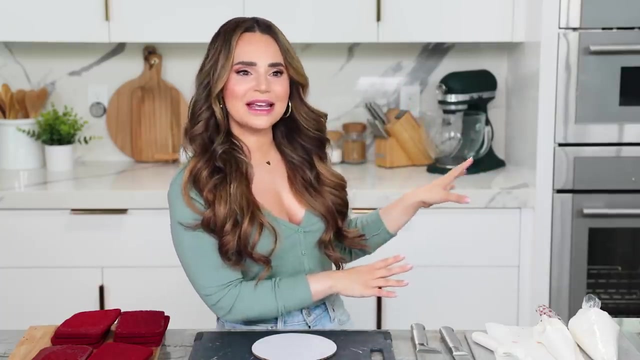 We're just. we're just, you know, crossing our fingers and hoping for the best, and sometimes that happens on your wedding day, A snag happens and you just kind of get through it, but we're committed. So that second tier is going to be strawberry. and well, she takes a break, you know, cuz she needs a minute. 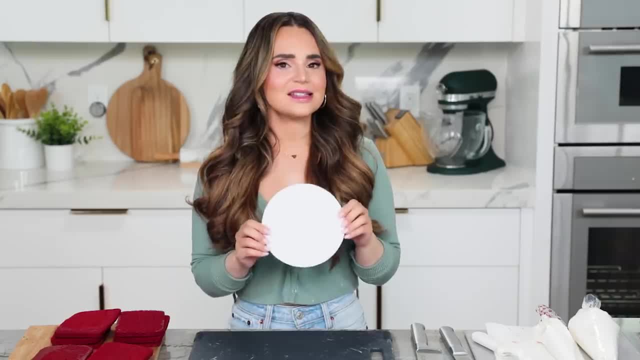 I'm gonna work on the top tier, which is our smallest tier. I think it's a six inch tier. I've got a little cake plate here and I'm gonna build on top of it and we're gonna move back to the red velvet and 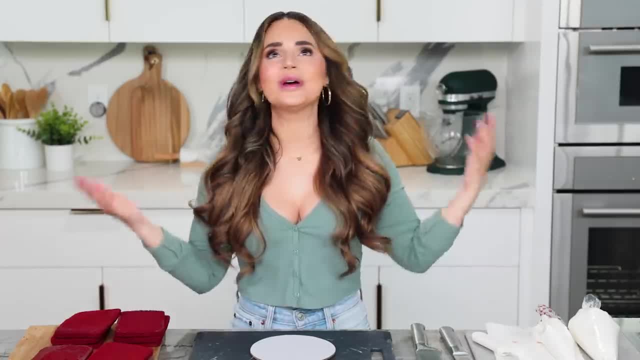 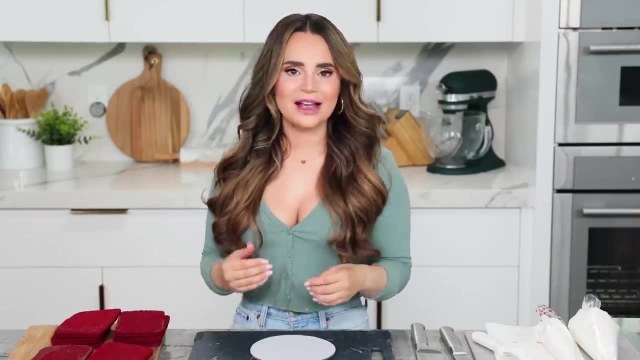 I did not know what I was doing when I was making this video, and if I could do it all again, I would only use the red velvet cake. It is Structurally more sound, it's more dense and it just works better. I'm gonna put a little icing here on the cake plate. 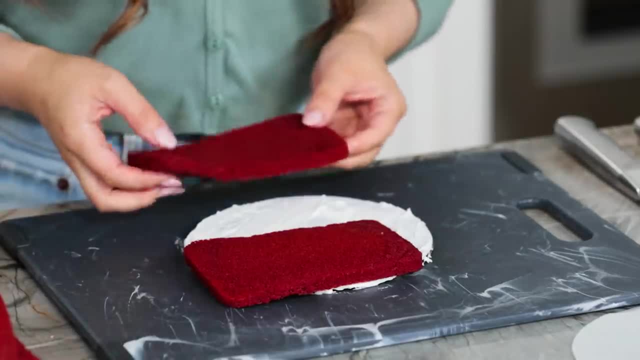 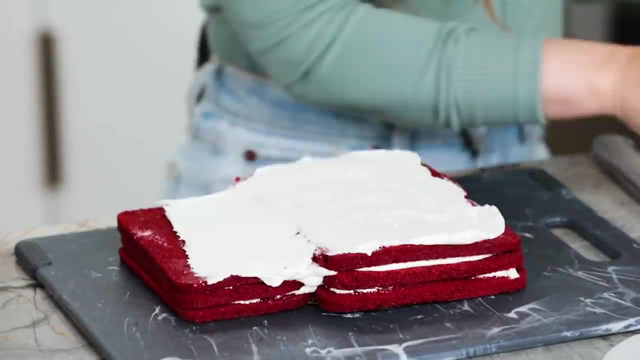 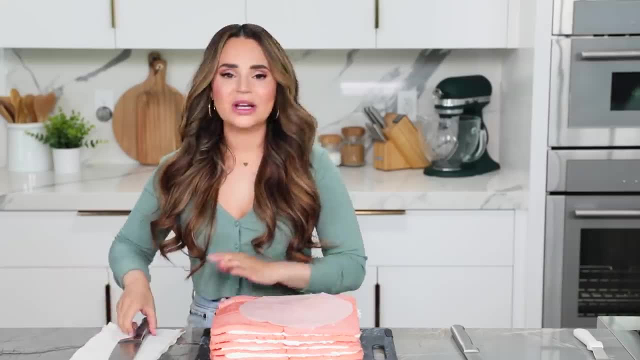 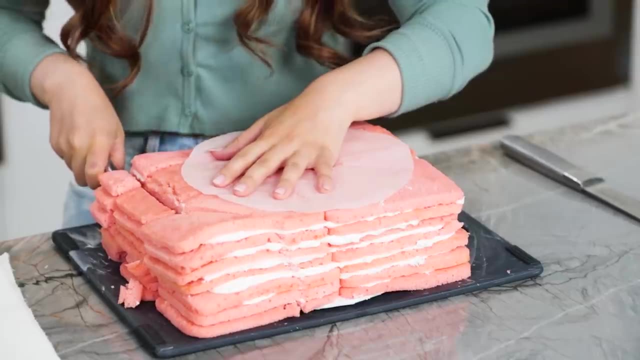 Still kind of a squishy hot mess, but we're gonna do our best to carve her, so I'm just Gonna start on the edges, like I did the other cake, and hopefully this is going to work. Let's take a look. even though she's squished, Oh gorgeous, I mean even though the texture is very. 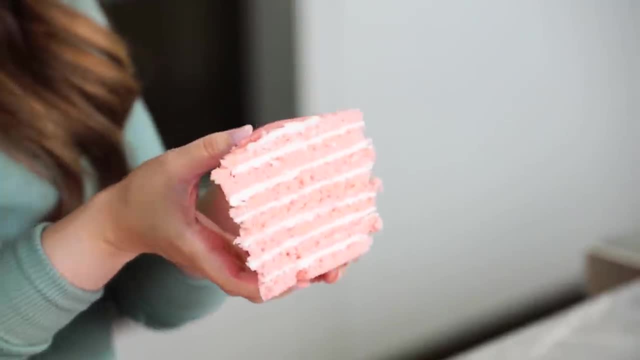 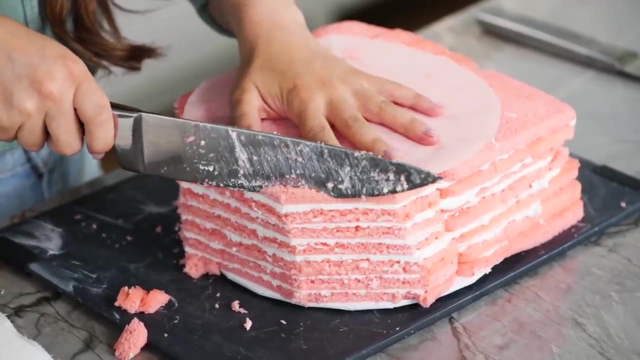 Squishy and delicate, beautiful cut. Look at that, Mike. Move this over, because I can see the edge is right there And we're just gonna try to follow it without it falling apart. might be a little bit smaller, That's okay, This is working okay. 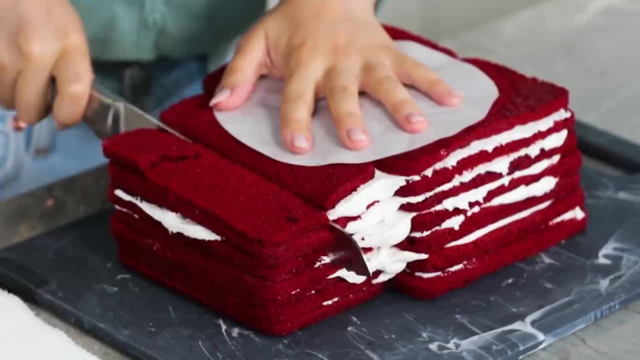 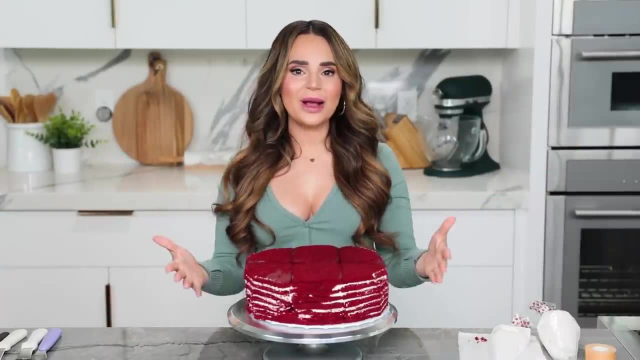 and I'm just gonna keep carving the cake until until it's more circular, And once I'm done carving this cake, I'm gonna carve the smaller cake. The cakes are carved, and now it's time to ice. I'm gonna start by icing our biggest tier first. 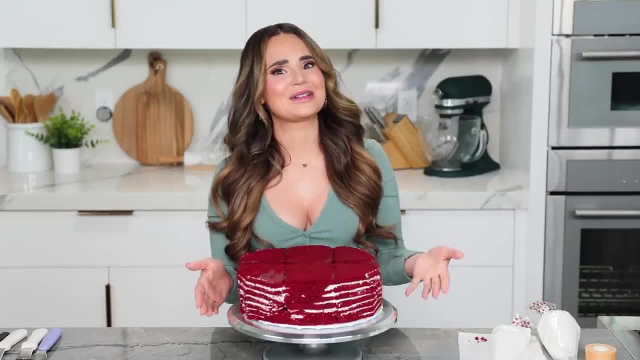 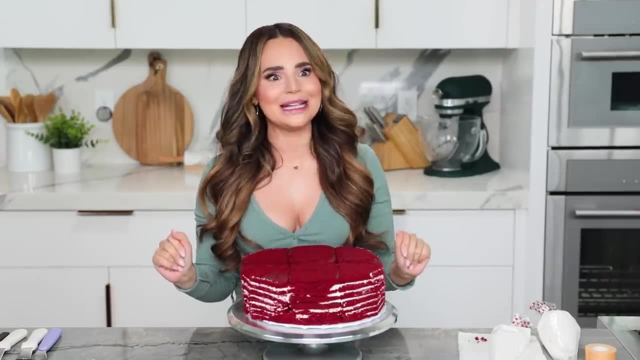 I've plopped it on top of a turntable to hopefully make this a little bit easier, And I'm gonna be icing a few layers on each tier because it's very crumbly, All right, so I've just got some buttercream icing over here. 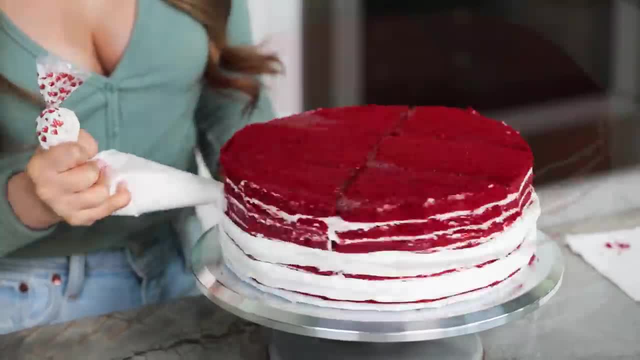 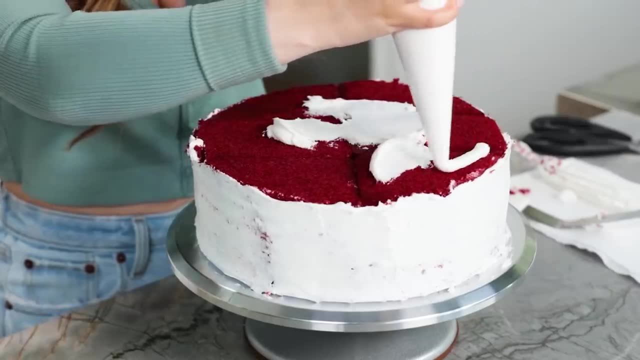 I'm gonna start at the bottom and work my way around. I'm gonna ice a thin crumb coat layer on. first. This is the most delicate I've ever iced a cake, because structural integrity is sensitive. After I get this crumb coat on: 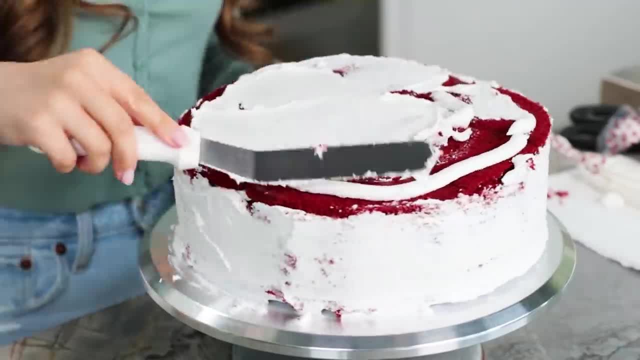 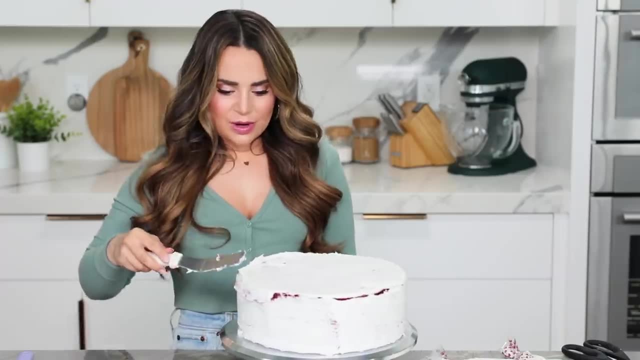 I'm gonna put a crumb coat layer on all of the tiers, let them chill for a second and then we're gonna put on the pretty layer. It's a little uneven but I can even that out with icing, So I'm not so worried about that. 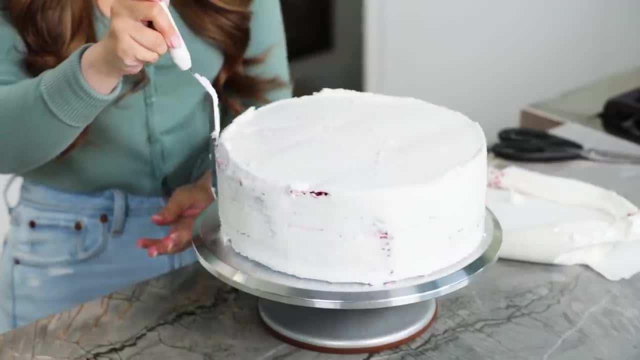 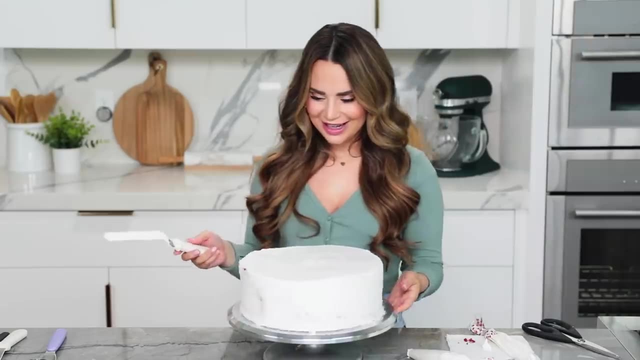 I'm just really trying to be gentle. You're so pretty, just stay together. Okay, I'm not mad about it. We got our crumb coat. It's looking crummy, just like it's supposed to. I'm gonna let this chill. 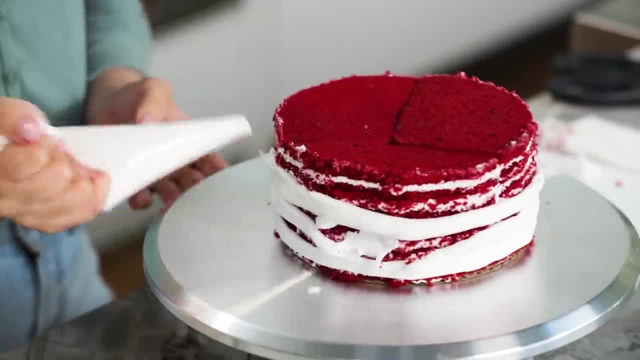 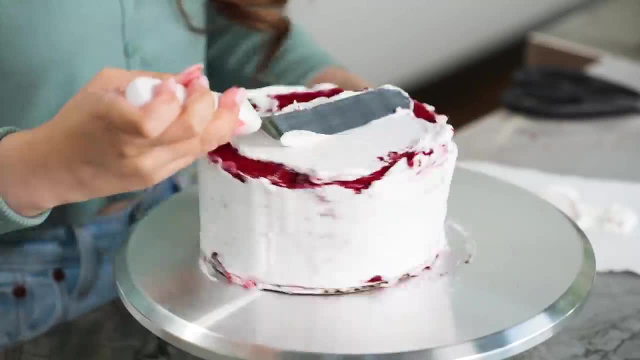 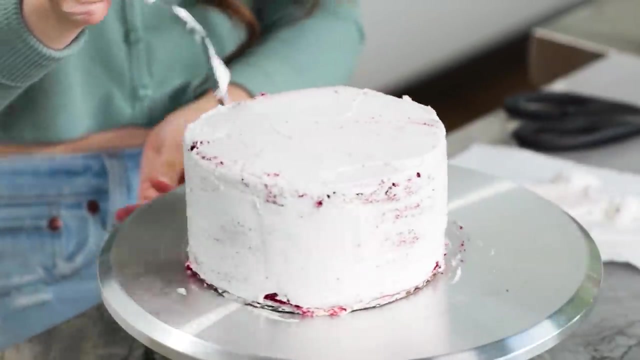 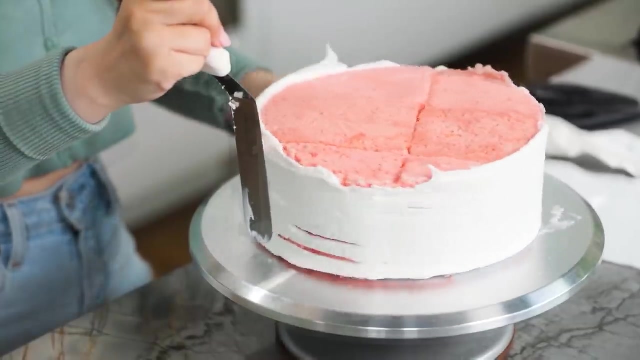 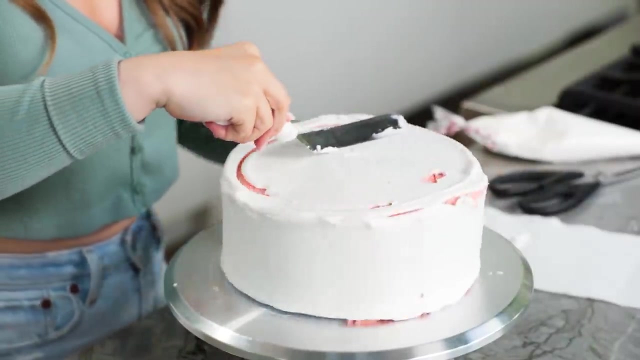 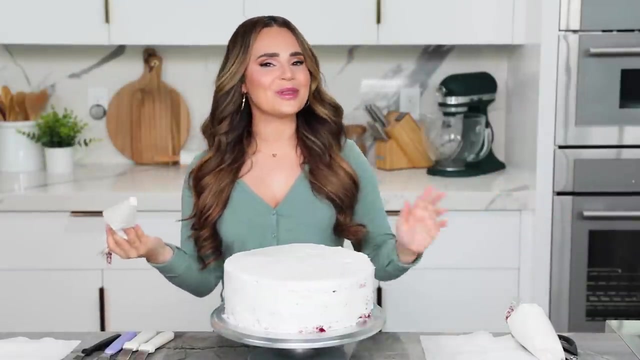 and then do the same thing to our other two cakes. Here goes nothing. We got our crumb coat and now I'm gonna put on the pretty coat, the top coat. I've decided that this wedding cake is going to be rustic and classic. 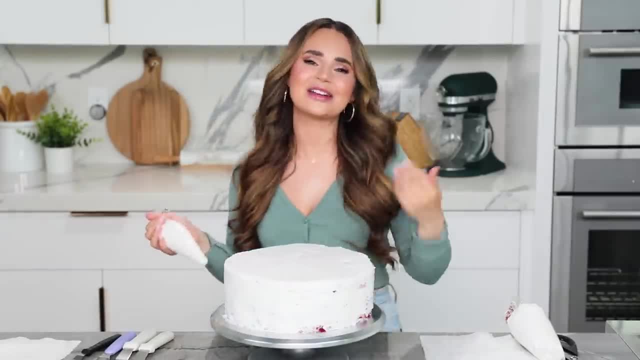 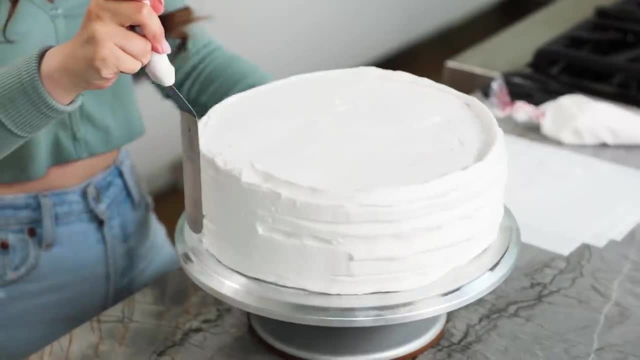 Rustic- because that's what the icing's gonna look like- And classic. I'll add a little decorations For the pretty layer. we're just putting on another coat of icing and I'm gonna try to cover all the crumbs. Okay, no crumbs. 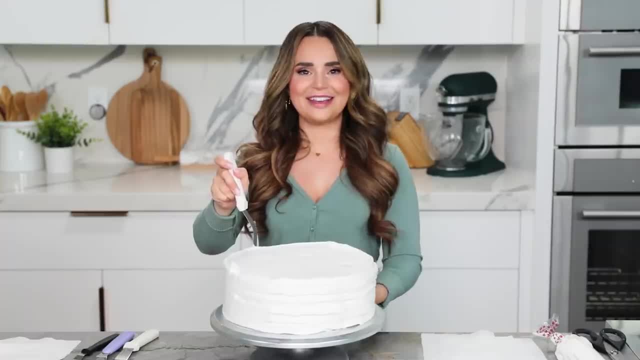 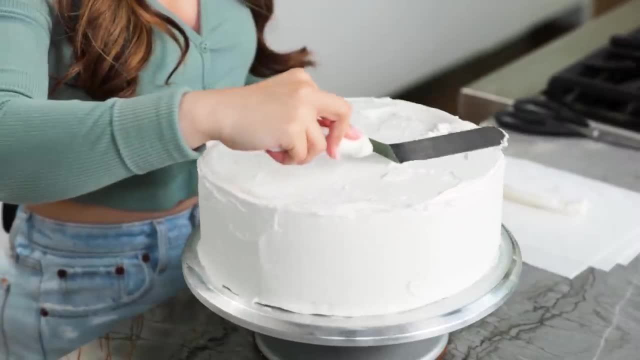 That's what the goal is. And if not, remember you guys, it's rustic, Not quite a naked cake, but maybe it will be Got pretty dang good Ice. the top Gotta cover all the crumbs, cover all the crumbs. 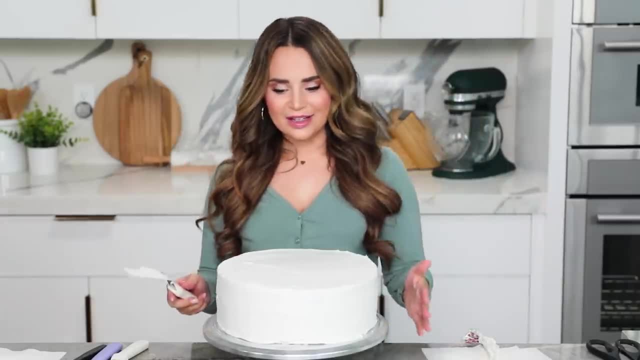 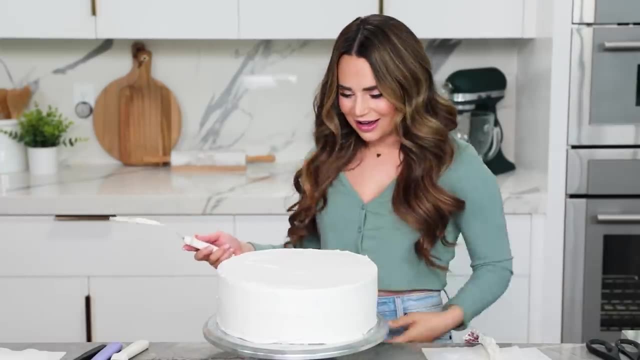 cover all the crumbs. What crumbs? Normally I would spend a while perfecting this, but I'm trying to get this wedding cake done by the end of today, you know for a wedding. So now to give it a little rustic design touch. 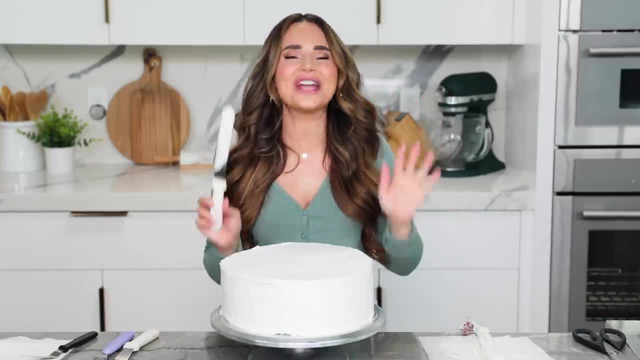 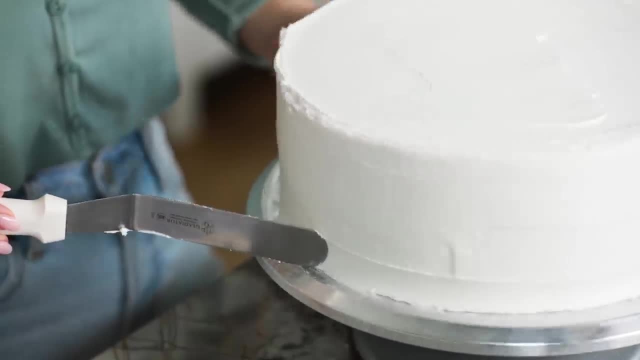 I'm gonna be using the end of my spatula and ever so gently making rings around the sides of the cake, Like so you just place down and really gently push and go all the way around The turntable really helps. It just gives you that control. 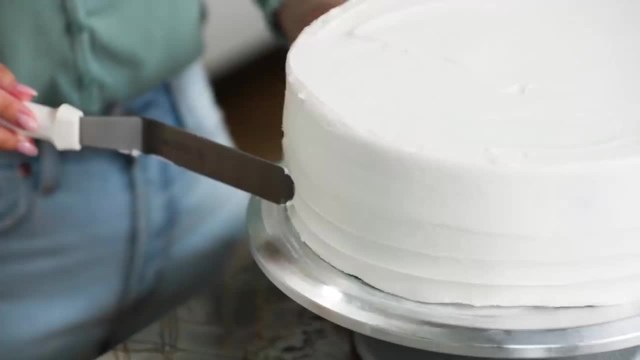 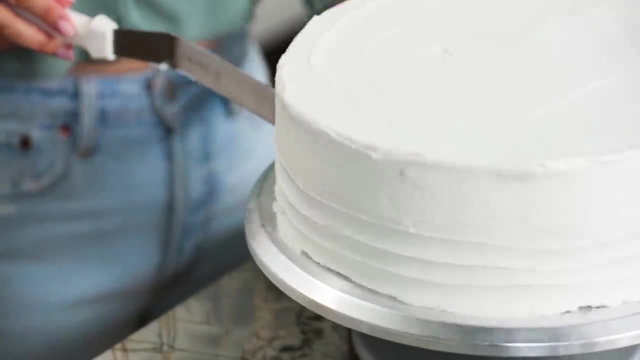 And I don't wanna take off too much icing and now I'm just gonna go up, go all the way around. The lines are not supposed to be perfectly even. They're supposed to look rustic. I think that's the best way to go with this cake. 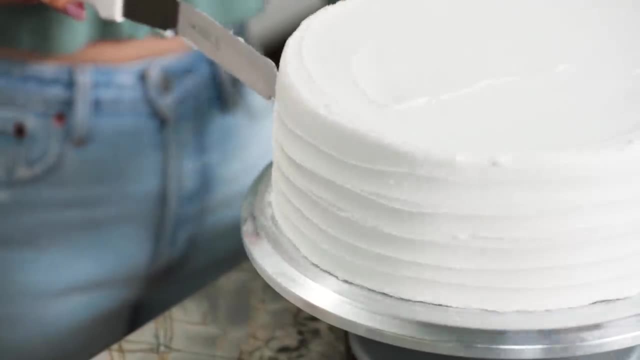 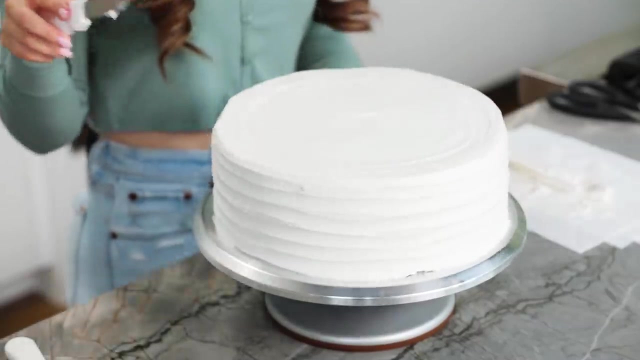 Rustic's great because if it gets a little messy, it's like it was designed to. Oh my God, they're so pretty. I'll do a little swirl up here too. Boom, my cast is done. Oh gorgeous, Love it. 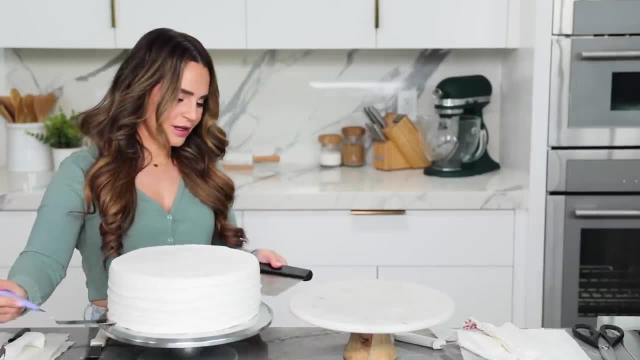 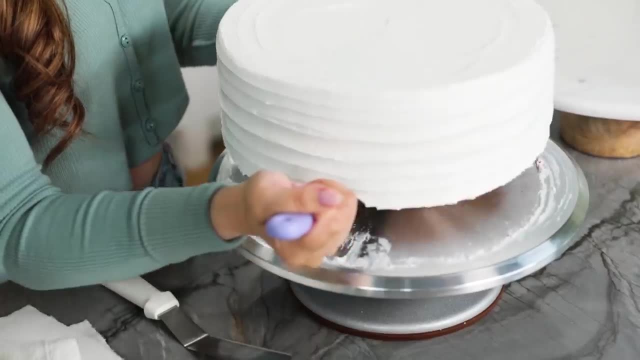 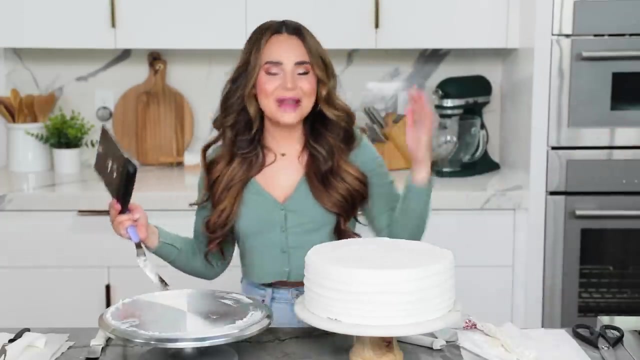 Okay, now I just gotta transfer it. I'm gonna tuck right under here, tuck right under here. You just gotta be fearless and just go for it. you know, Boom, I think this is the biggest cake ever made in an Easy-Bake oven. 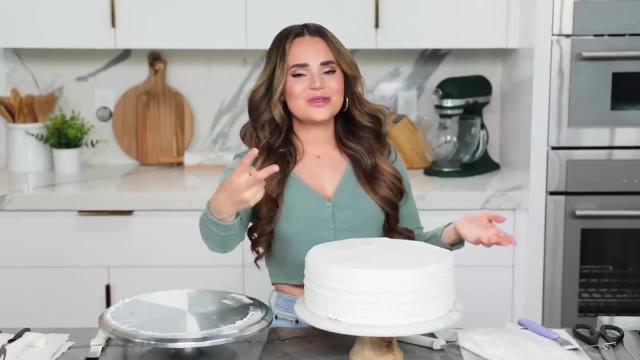 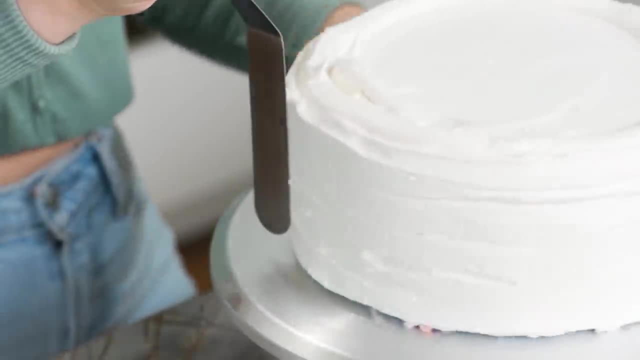 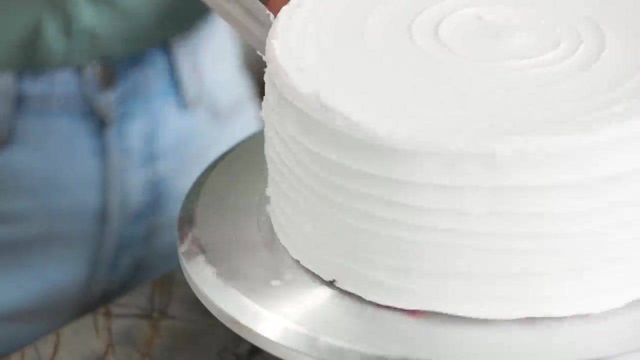 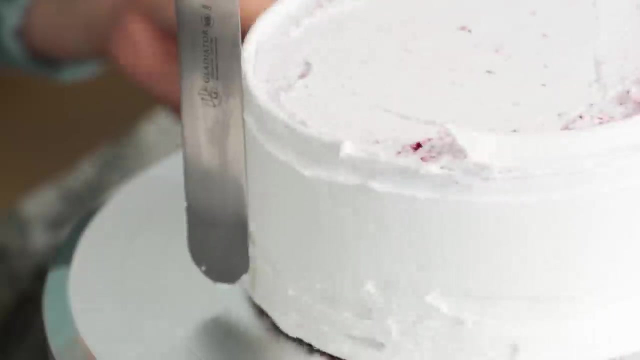 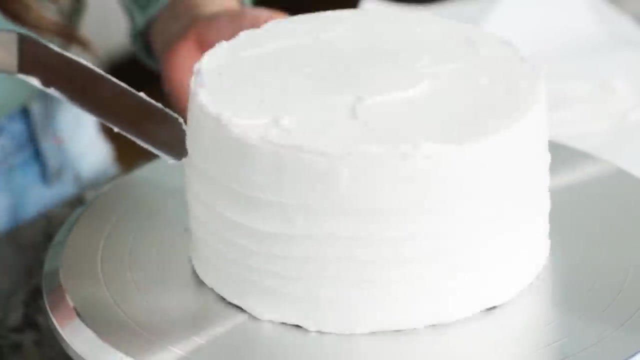 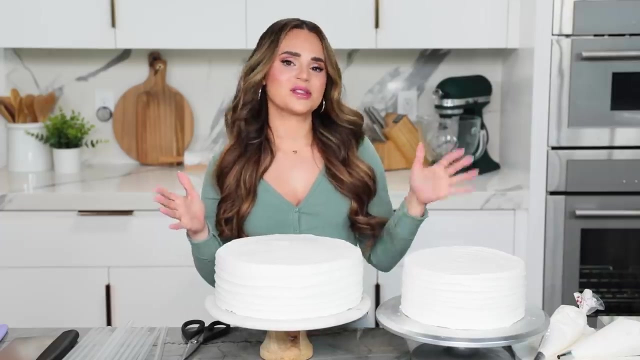 But I'm not saying it was the most, but I think it was the biggest cake ever made in an Easy-Bake oven, But Think we could go bigger. now I'm gonna ice the other two tiers. in the same way, When putting together tiered cakes, you always want structural support. 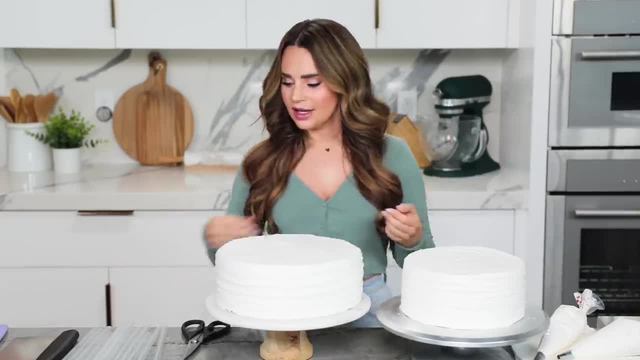 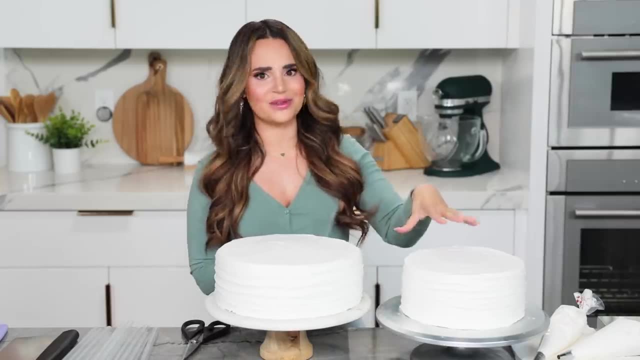 And that's why I put cake plates on the bottom of each tier, because you're gonna put these little jobbers In between the layers to help the cakes not sink into each other, especially because this cake is very squishy. I don't think she could handle much today. She's very sensitive, So what I'm gonna do is 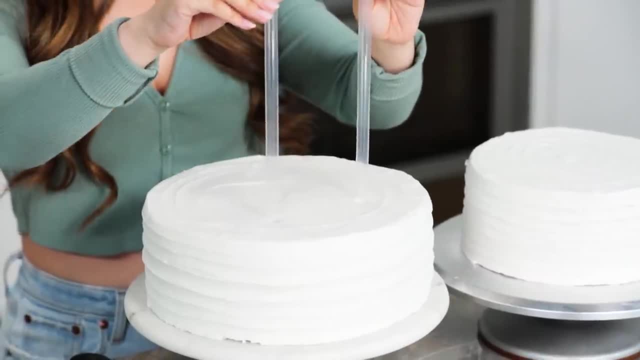 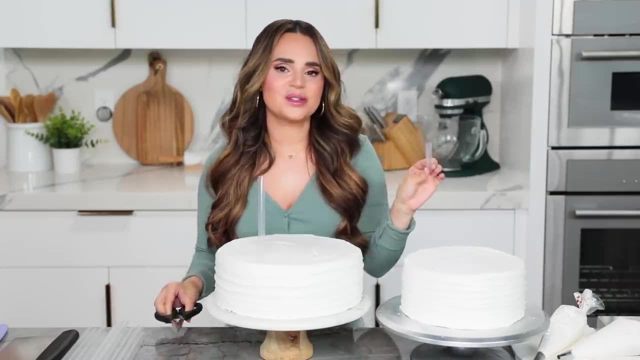 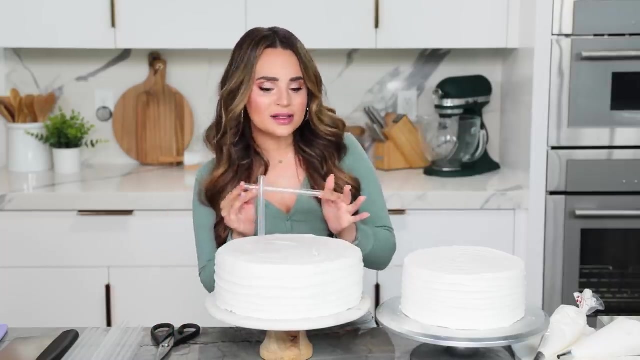 Eyeball it. I'm gonna place a lot of these into our big cake And you push them down and then you pull up just a little bit and then cut. I'm using boba straws because I have a bunch of these around the house, But for cake dowels you can use just about anything. they have plastic reusable ones that my mom uses. 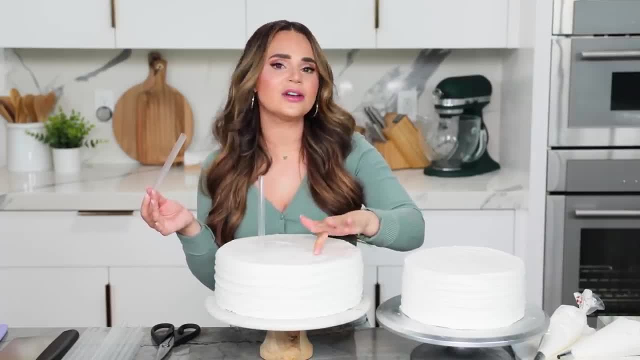 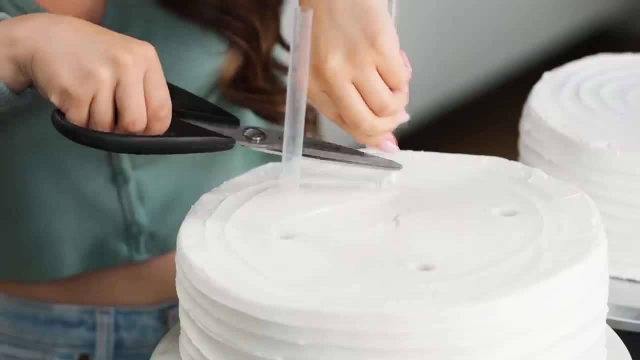 They have wooden dowels. So whatever you got in your kitchen, you can even use straws. you know, I'm just gonna need a lot of straws. Okay, let's put a bunch of these in. Usually, I just put in five. Today not so much. We're putting in a bunch. 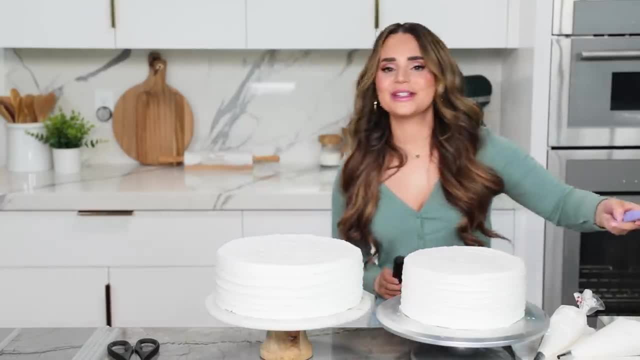 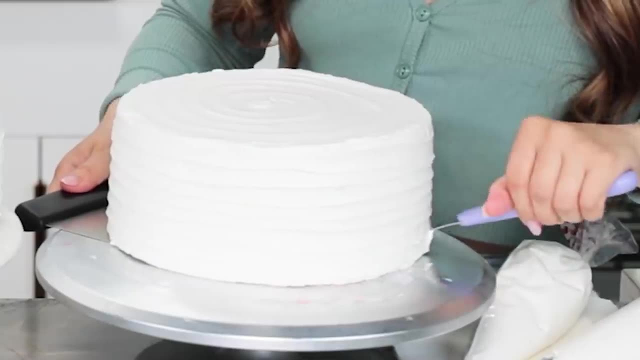 Okay, hopefully she'll hold up. now the terrifying part: transferring a cake. I usually use one of these Offset spatula. get it on there. Oh gee, She's moving. Oh no, I went too far. Oh gee, I went into the cake. 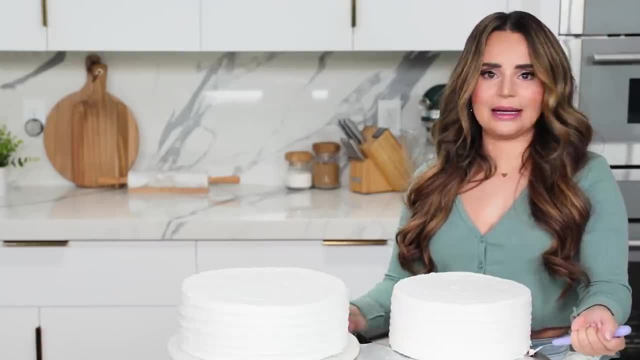 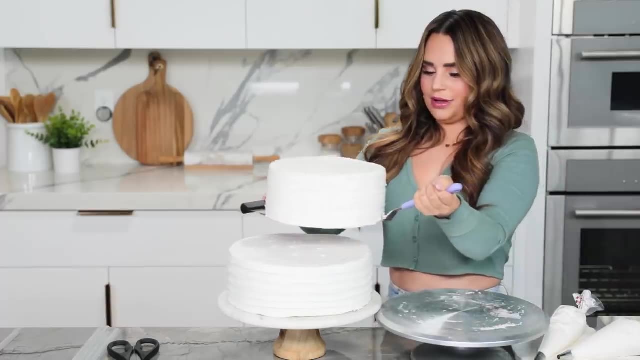 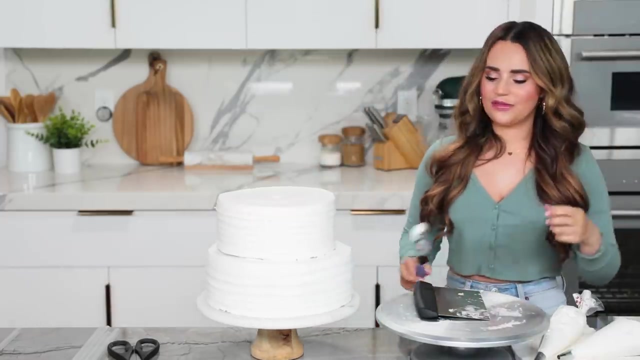 This is not good. No, we got this. Okay, I'm gonna put the ugly side back here, because we have now have an ugly side. Oh gosh, whatever I do, don't drop this. Put her down. Whoa, Yes, you just have to fill in a little icing here in the back, but other than that, 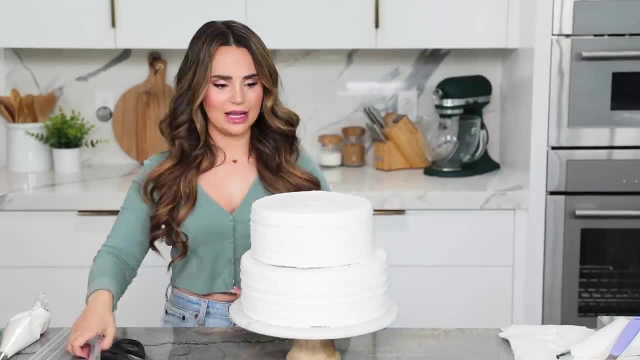 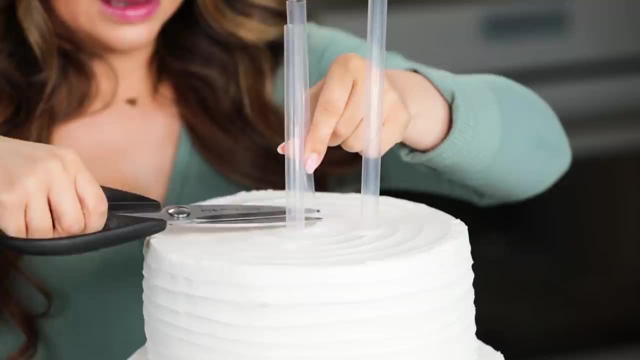 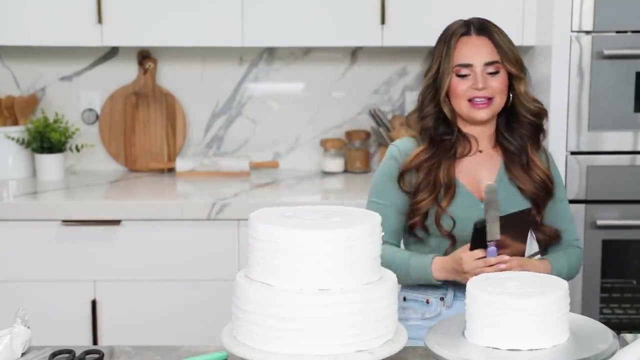 Like. I did it. I'm proud. Okay, Now we just need one more. Okay, for our last. here again, We're gonna put in a lot of structural support here at the top. I need a steady, sturdy cake. Whoa, oh geez, here we go. I'm gonna hype myself up. Whoo, We got this, got this go underneath and we're up, and we're up, and. 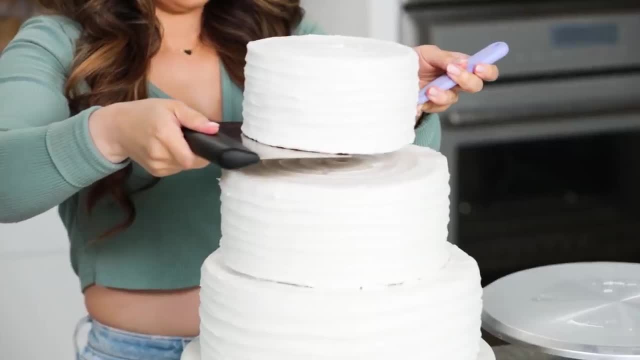 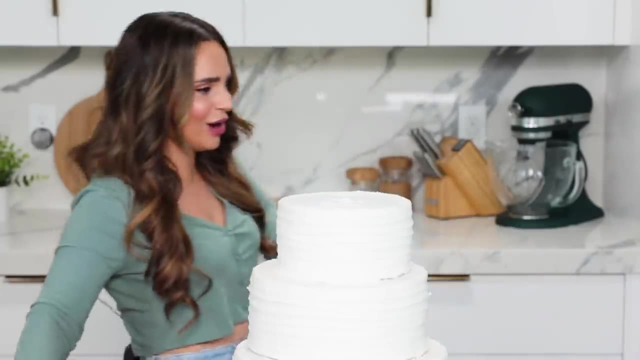 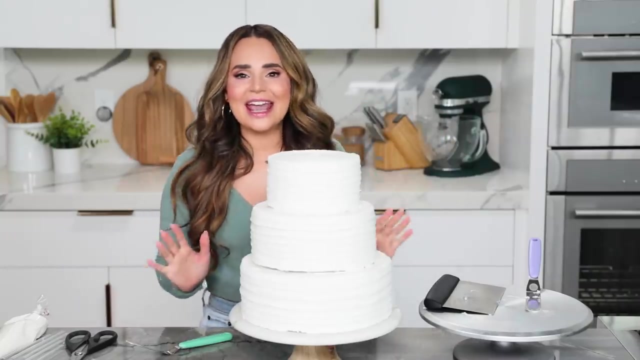 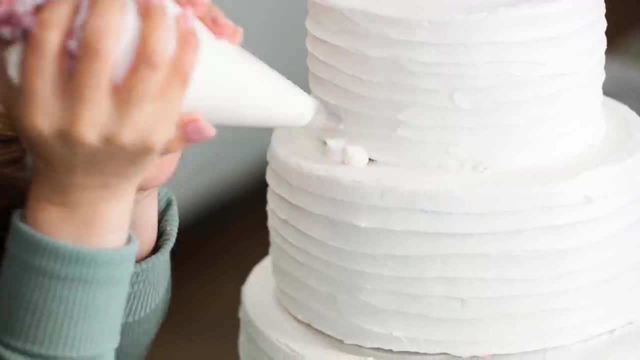 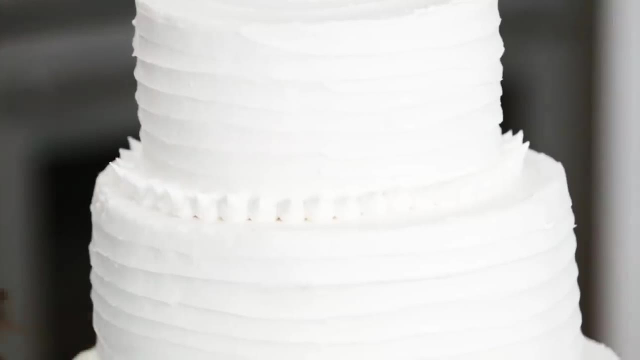 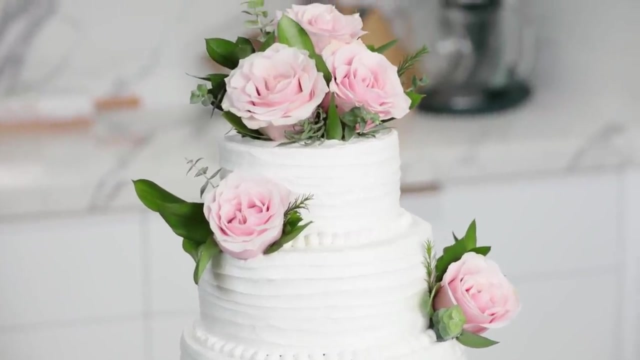 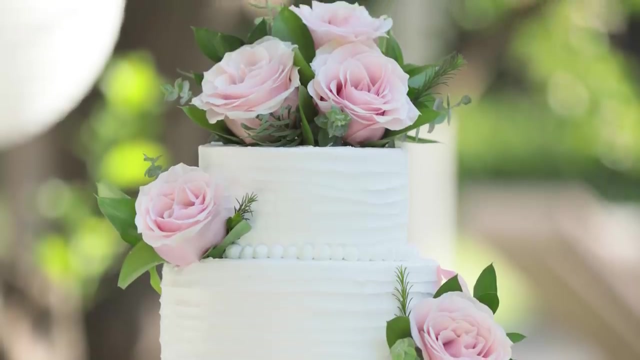 And I'm gonna add some flowers. And Here is the wedding cake that I made in an easy bake oven. I cannot believe this actually worked. it did take a while. It took a lot of time to make all the little cakes and put it together, but it's awesome. 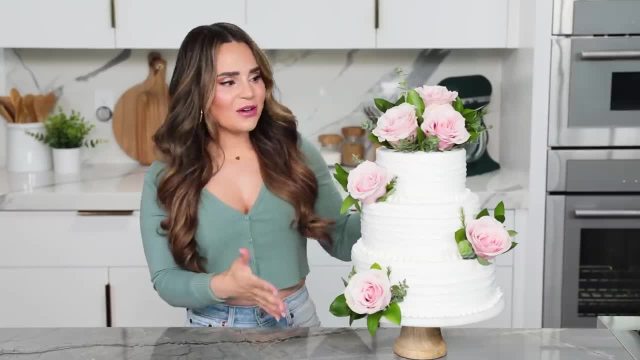 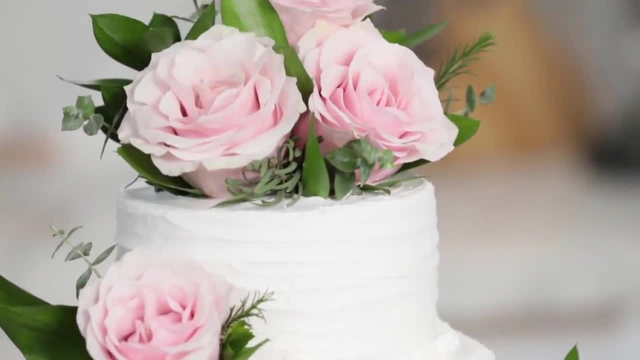 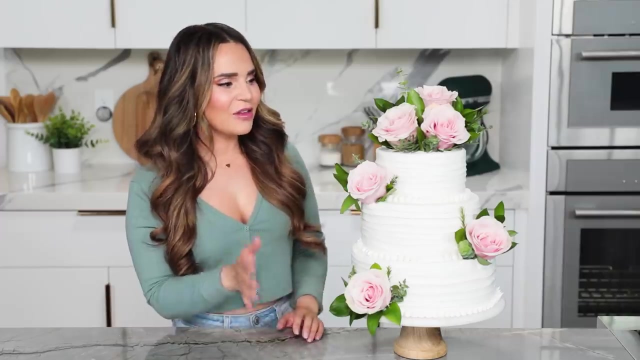 I'm like kind of shocked that this is holding together for decoration only did was get some flowers at the store. I love roses. my name, Rosanna, means Graceful rose. they're my favorite flower and I think that they're so romantic, So I love seeing them on wedding cakes. now, these flowers are a little larger than I was hoping. 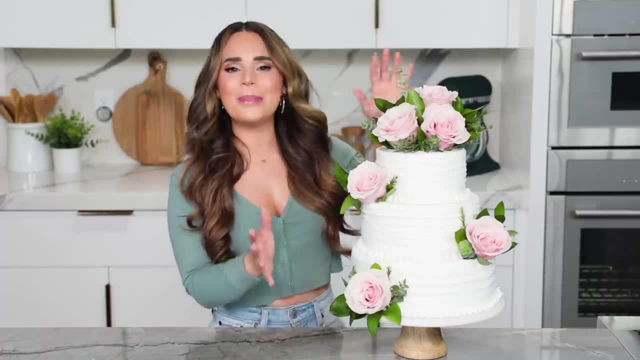 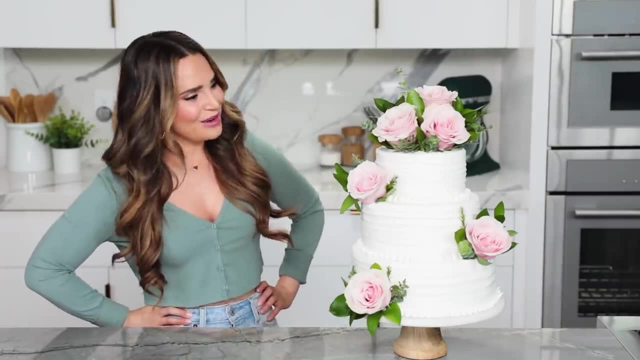 But this is all they had at the store, So the roses are a bit big for the cake. but I gotta say this is a cute rustic cake. It is not bad. my mind is blown. I didn't know if this is gonna work or not, and it's actually holding up. 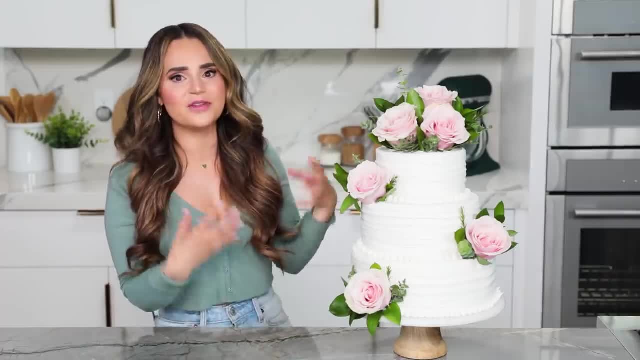 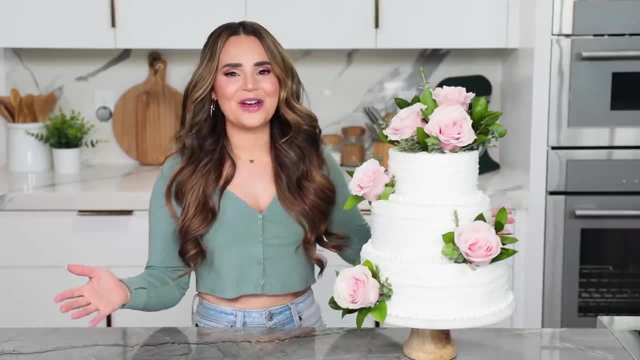 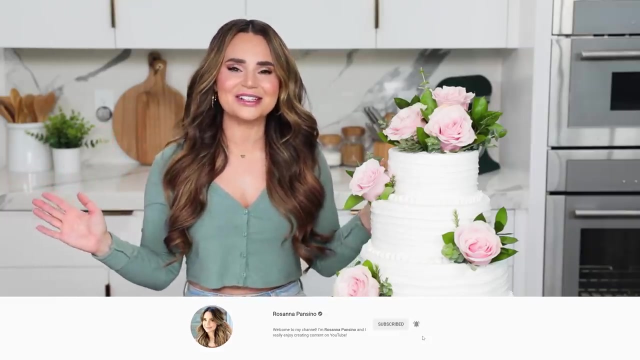 I had a lot of concerns about the strawberry layer because it's Very soft. I'm obsessed. We did it, mom, look. Anyways, this was so much fun. Thank you all for watching. if you enjoyed this video, Please give it a thumbs up, click subscribe and ring the bell to receive notifications every time I post a new video and 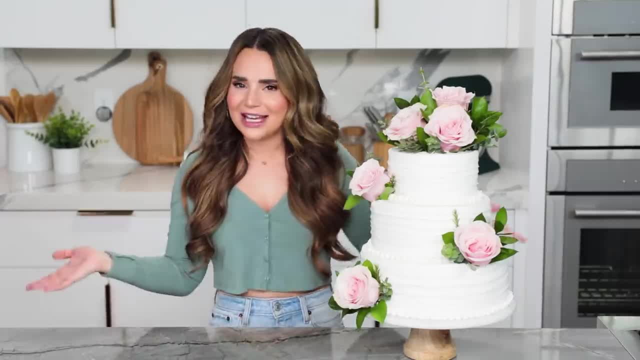 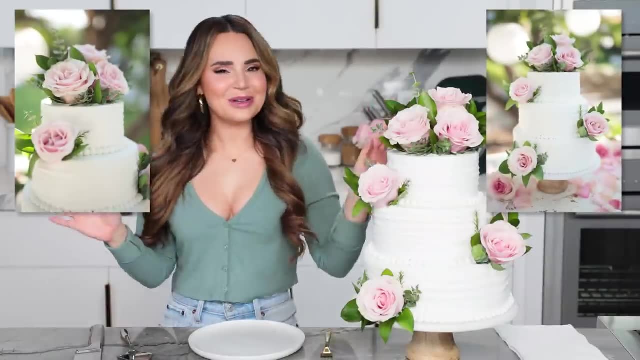 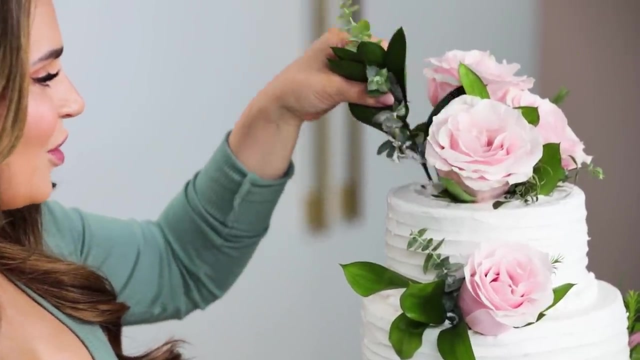 Please let me know in the comments down below What video would you like to see next, because I am trying a whole bunch of fun Things. this year. I took some cute pictures and now I get to have a slice. Let's give this cake a try. I've got to move some of this cute little topper right here, and here we go.